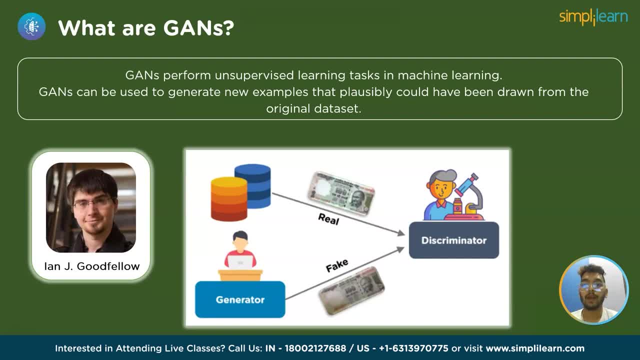 So this is an image of GAN. GAN is a database that has a real 100 rupee node. The generated neural network generates fake 100 rupee nodes. So the discriminator network will help to identify the real and the fake node, Or the real and the fake images you can see. 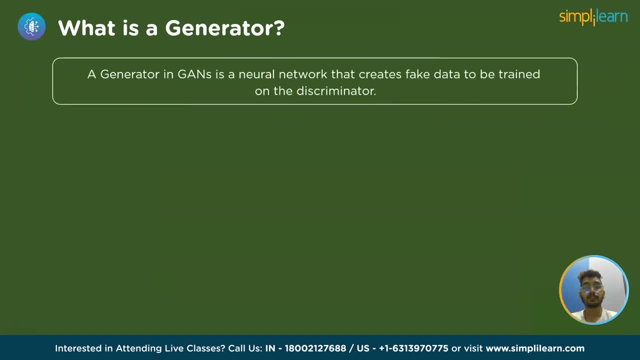 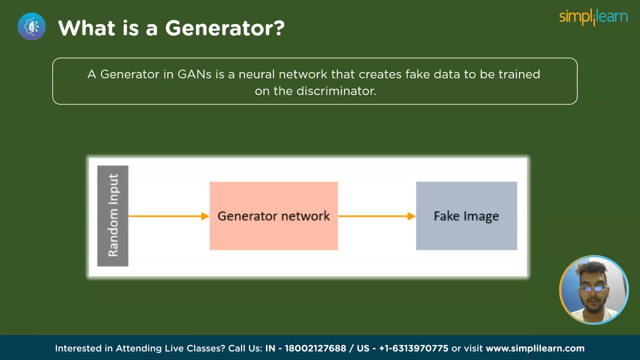 So, moving ahead, let's see what is a generator. So a generator is a GN neural network that creates fake data to be trained on the discriminator. It learns to generate plausible data, So the generator examples or instances become negative training examples of the discriminator. So 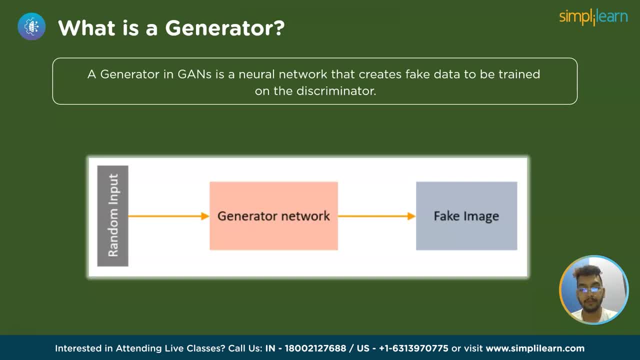 as you can see here, the random input generator- new fake image. The main aim of the generator is to make the discriminator classify its output as real. So the part of GAN that trains the generator includes the noisy input vector or generator network which transforms the random input into instance, or the disciplinator network. 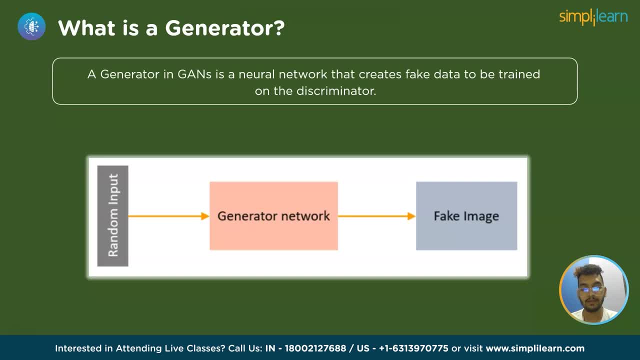 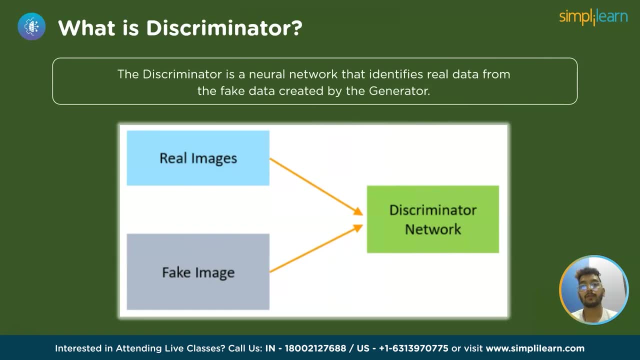 which classifies the generated data. So after seeing what is a generator, let's see what is a discriminator. So discriminator is the neural network that identifies the real data created by the generator. so the discriminator training data comes from two sources. the real data instance, such as real pictures of words, human currency, nodes and anything, are used by. 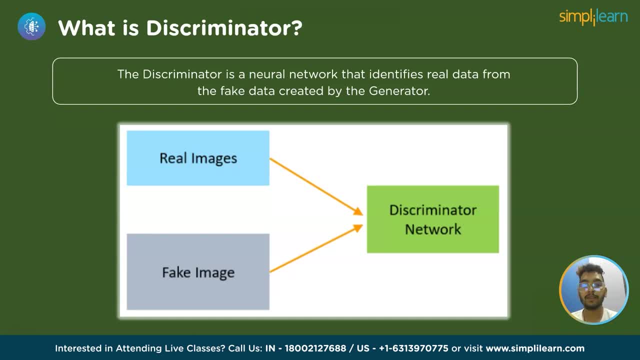 the discriminator as a positive sample during training. the second one is the fake data instance created by the generator are used as a negative examples during the training process. so discriminator decide from the real images and the fake images generated by generator and discriminator decide which is fake and which are real. so now let's move on to the programming part and see how we can. 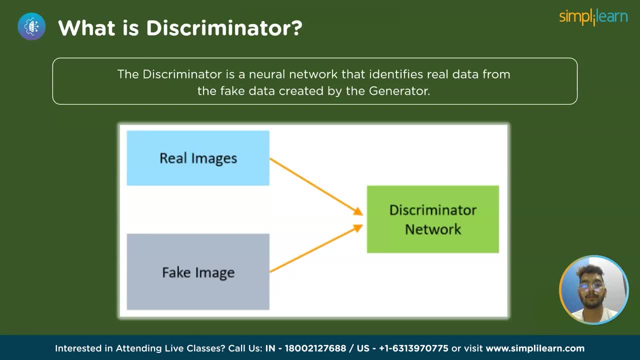 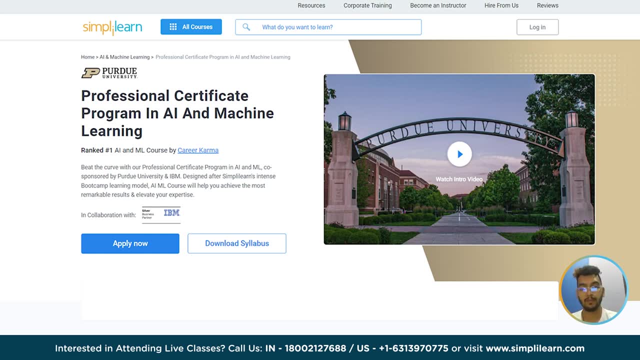 use gan using celebrity face image data set. so before move on to the programming part, let me tell you that the demand for machine learning ai is growing faster than that of other profession. in fact, according to statistics, there will be more than 2.3 million job opening in the field. 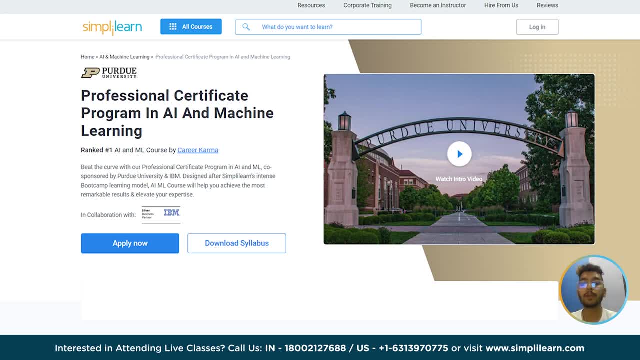 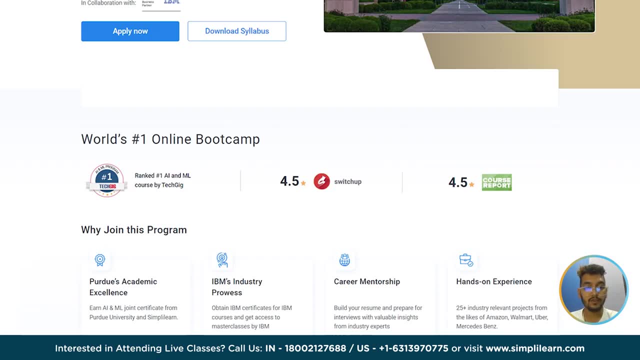 of artificial intelligence and machine learning by 2023. but you can beat the curve with our professional certificate program in ai and machine learning, co-sponsored by purdy university and ibm. this course covers tools and techniques like numpy, pandas, python, sci-fi, along with industrialized machine learning and machine learning and machine learning. 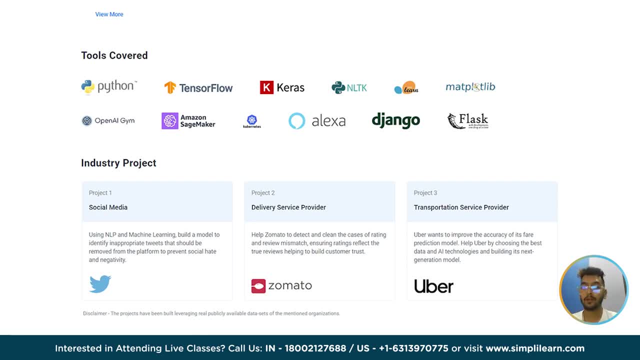 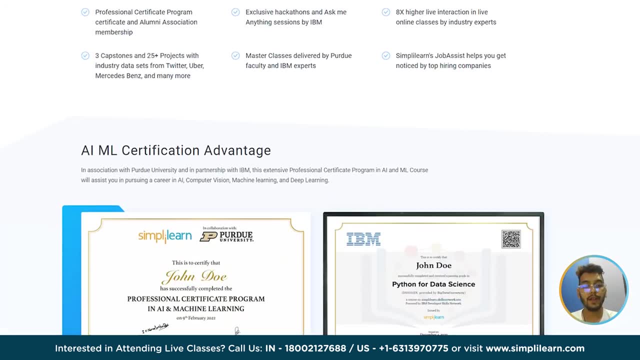 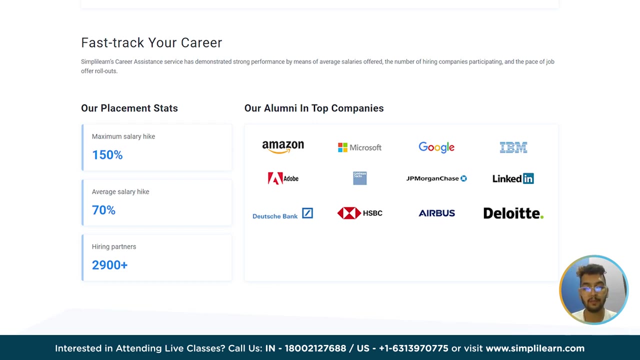 projects like social media by twitter, delivery service provider by zomato and transportation service provided by uber, and many more amazing projects. choosing this course, can you get hired in renowned companies like netflix, amazon, facebook and adobe, and many more, and an average salary hike of 70 percent. so what are you waiting for? join the professional certificate program in ai and 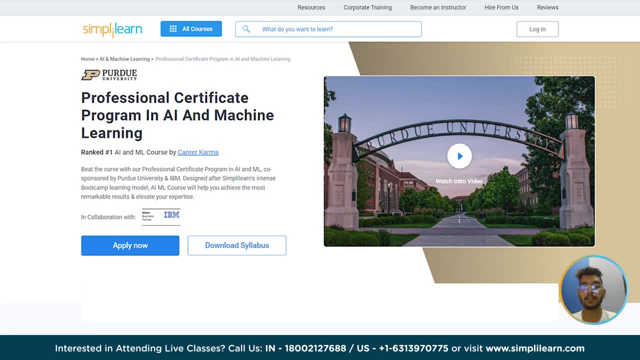 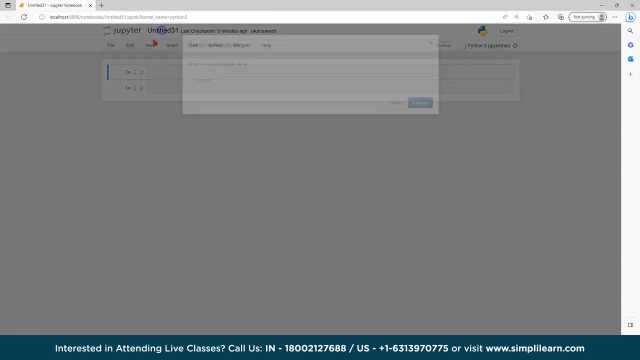 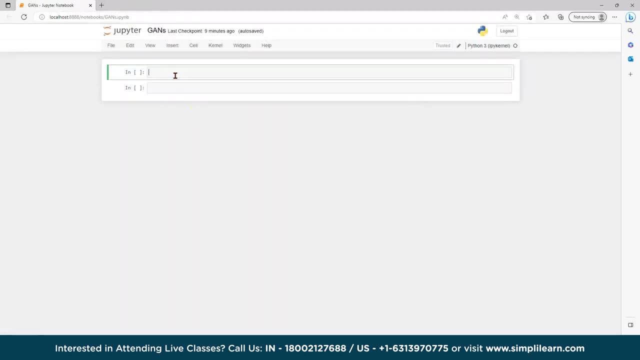 machine learning and excel your career into machine learning. the link is in that description box below. so here we will start with gan: generative adversarial network. okay, so first i will rename it gan. okay, so here we will import, uh, some libraries like import os. so we will do from pytorch machine learning deep learning library. 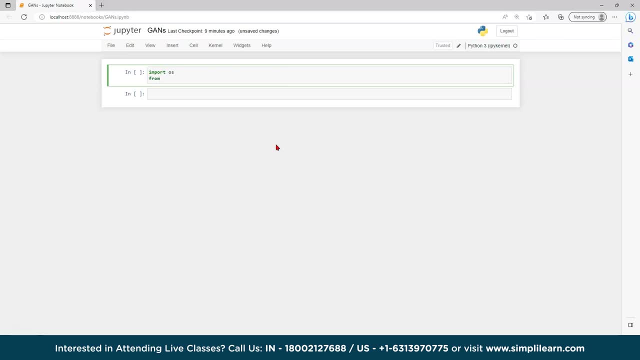 which work for like neural networks. so here i will like from torch dot utlis dot data import data loader. okay, so what is this torch dot utlis dot data? so there's the apst, get class representing a data set, and you, here you can custom data set that inherit data set and override. 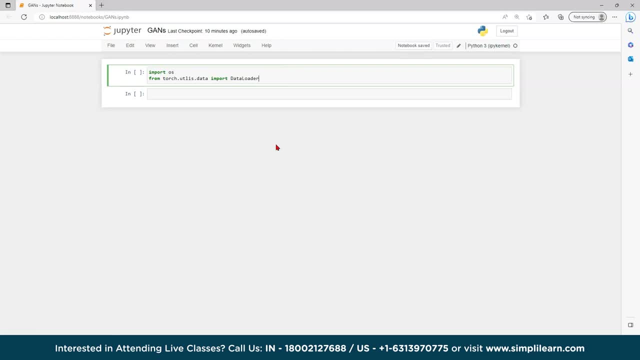 the data set. okay, and this import data loader. so data loader is a client application for the bulk import or export of the data and we can use it for to insert, update, delete or export and 거지 it available asенной talk about a five-翼 class for filtering data. layout in kanированastroniscom. 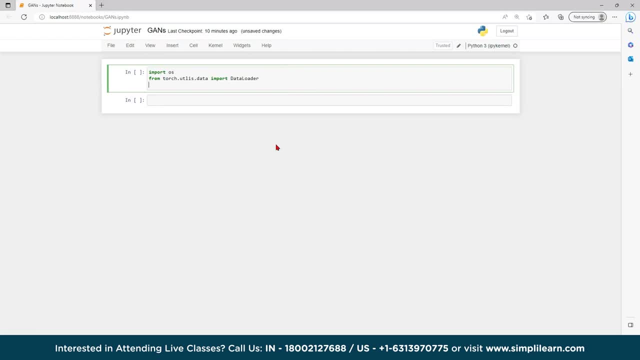 update, delete or export, like records. and when importing data, data loader reads, extract and loads data from the csv files, like comma separated values or from a database connection. you can say: and when exporting data it's output a csv file. okay, then moving forward, dot vision, dot transform. 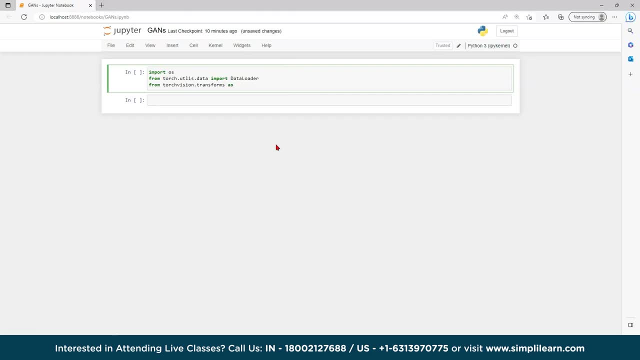 as t. okay, so transform are like very common image transformation available in the torch vision so transformation module. they can be changed together using compose. so most transform classes have function equivalent. functional transform give fine grained control over the transformations. and one more like from torch vision vision dot transforms. 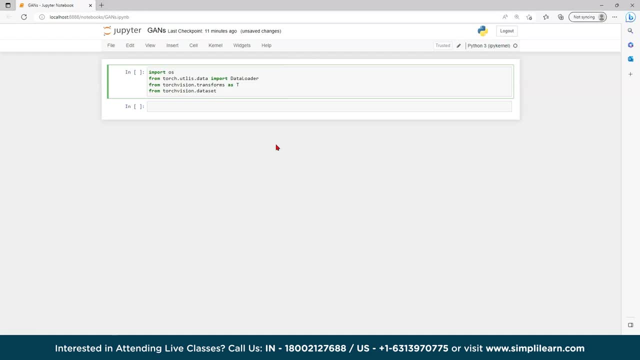 sorry, data set sets. import. import image folder. import image folder. import image folder. ok, invalid syntax. why it is invalid? let i will tell you. it's not, it's import. okay, yes, so now what i will do. okay, torch utils. it is out of the object. yeah, now it's working fine. so now we will import the data set. so we are here. we are using. 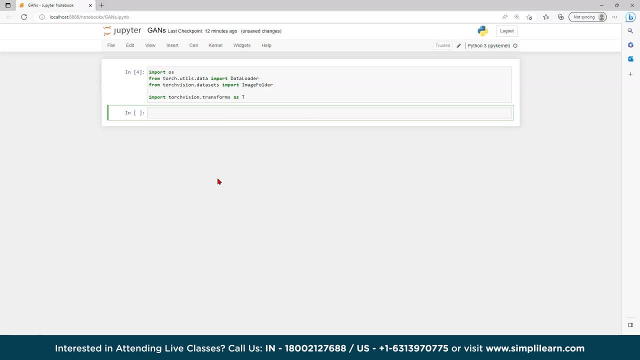 celebrity face image. okay, so i will provide you the data set in the description box below, don't worry. okay, so you can download from data set directly from there. so this is my path to data set on five desktop face image data set. okay, now let's run it. 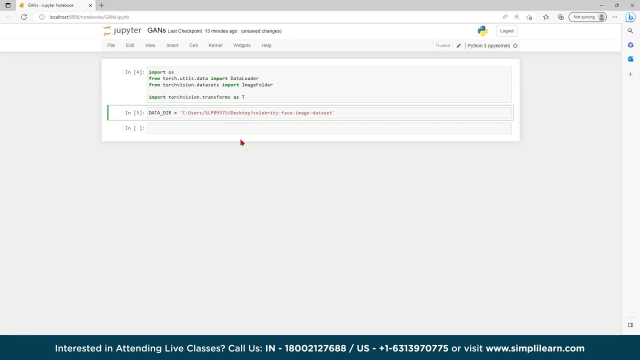 okay, now, let's run it. okay now. i guess it's fine. yeah, so here what i will do: i will set the image size and all. so image size: person 64. then bad size equals to 256.. then batch size equals to 256, then stats. 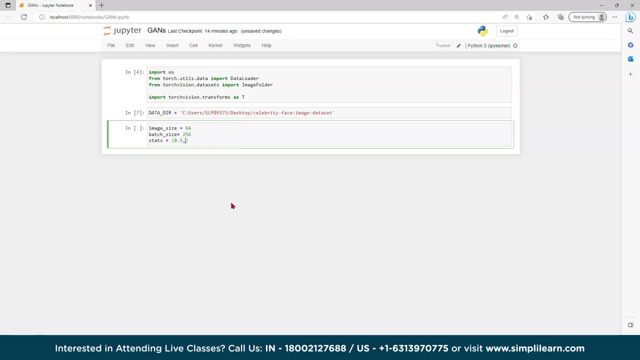 equals to 0.5 comma 0.5, and again stats equals to 0.5 comma 0.5, and again 0.5 and again 0.5. okay, comma 0.5 comma 0.5, comma 0.5. okay, so here we have set the image size and the batch size. 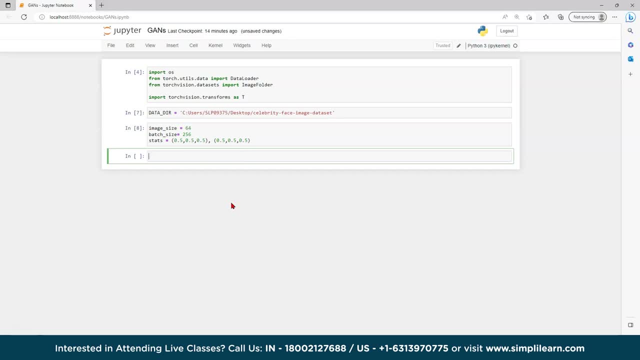 and the stat values. so now what we will do. we will train the data set. so here i will write train. train ds equals to image folder of data. sorry, data directory. comma transform equals to t dot, t dot compose. here i will write d dot g size, then image size. 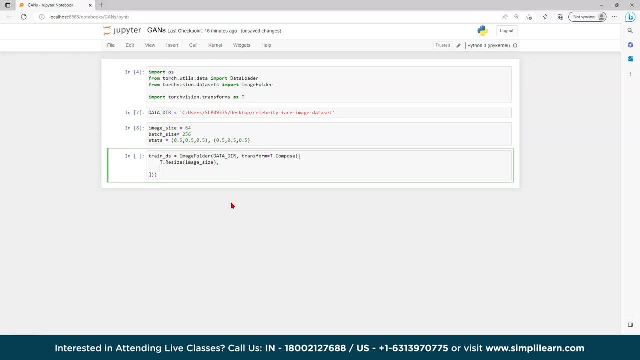 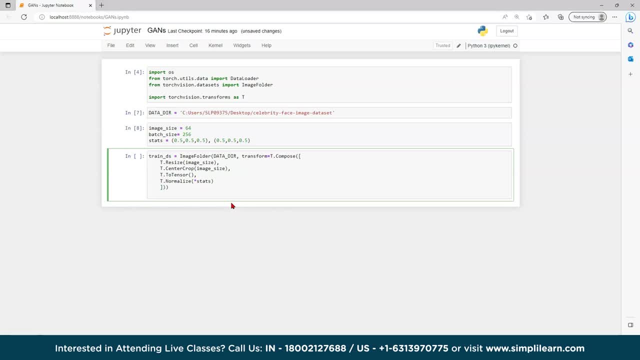 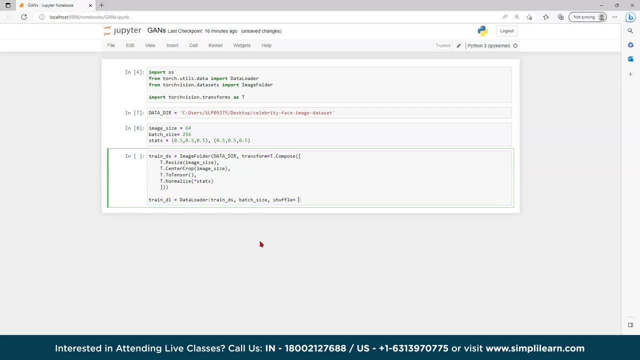 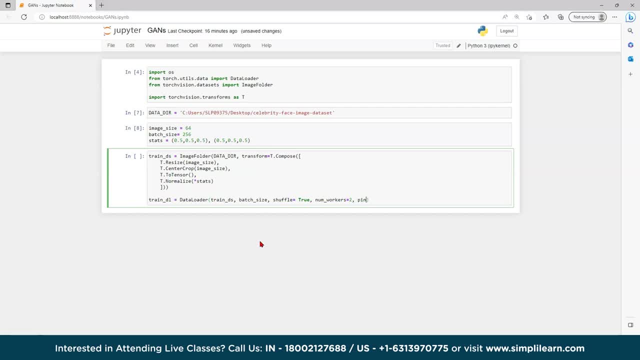 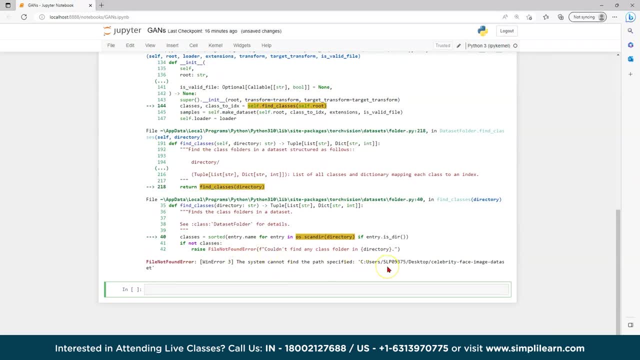 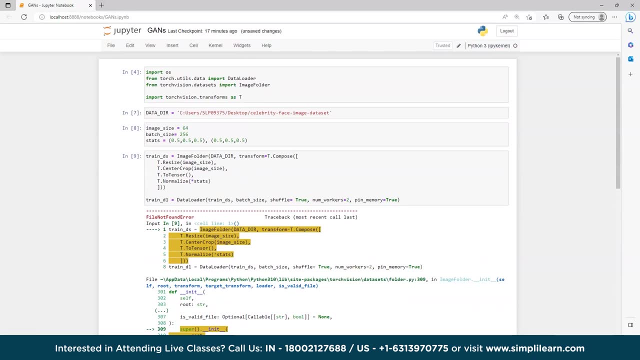 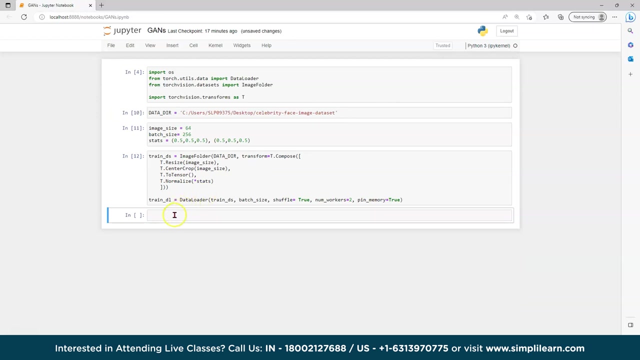 comma t dot normalize. comma t dot normalize. comma t dot normalize where see user. okay, so there is a path error. okay, so let me copy my path. let's see now. let me done. yeah, so it's working fine. so let me import torch from torch vision dot. 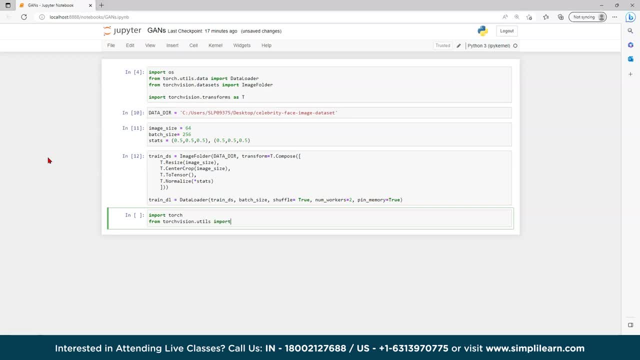 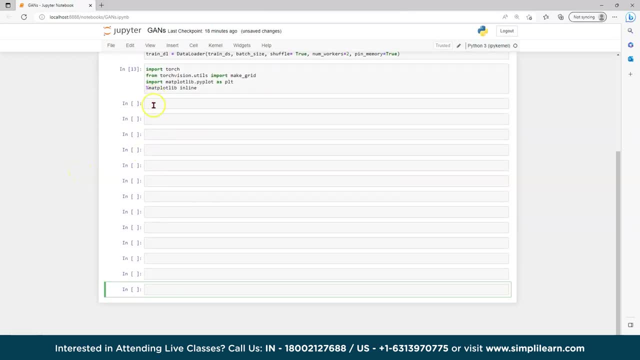 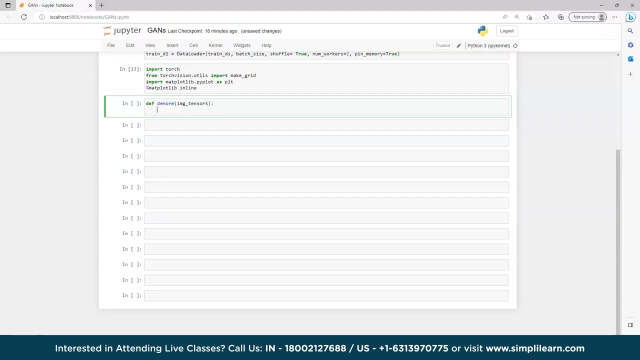 So here I will write now: make a function known img tensors, then return img tensors, stats one zero plus stats zero and again zero. okay, so let me run this now what we will do. we will make again a new function for show images and show badges. okay, for that I will write: 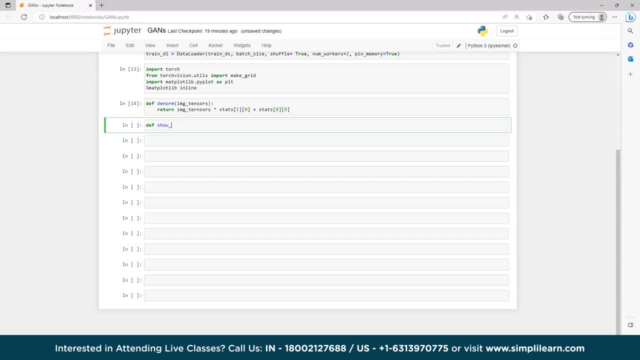 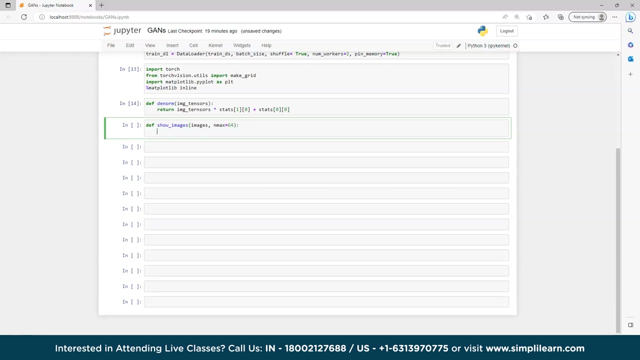 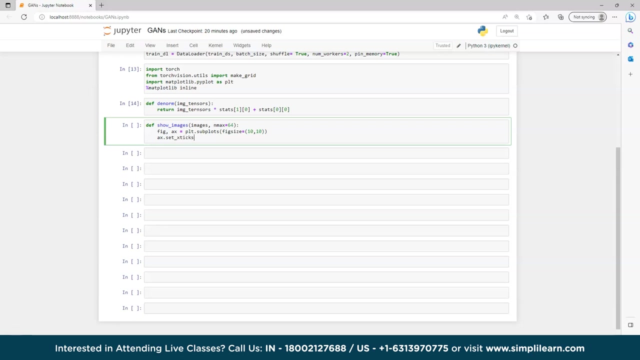 df- show df. show df. show image. Okay, then Images. comma nmax equals to 64: 64 will be there. then figure comma axis equals to plt dot subplots. figure size 10. comma 10. ok then ax axis: dot set x takes. ax dot set y takes. 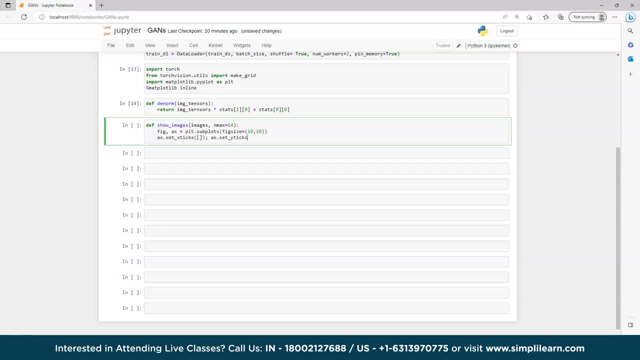 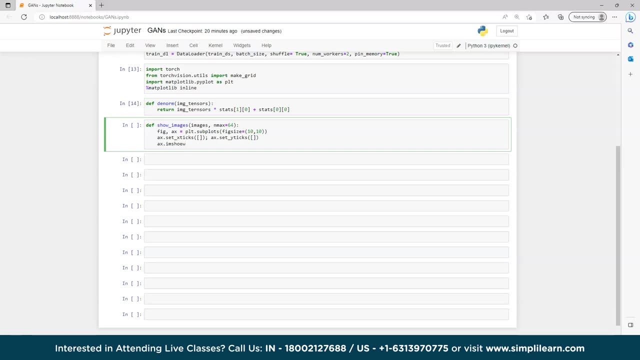 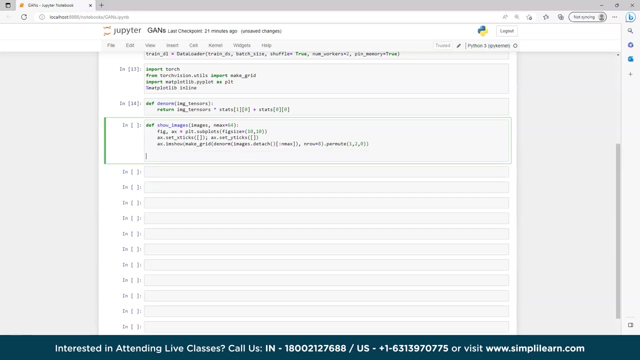 ok, then ax dot. I am show. this is image show. then make grid, the non, the non, function images, dot detect. and then and max comma and row number of rows will be 8. then dot permute 1 comma, 2 comma, 0. ok, then d here. 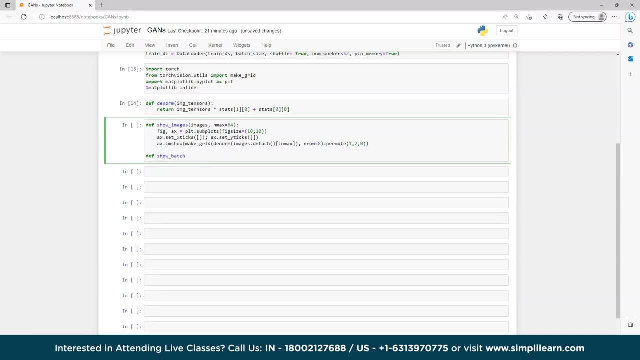 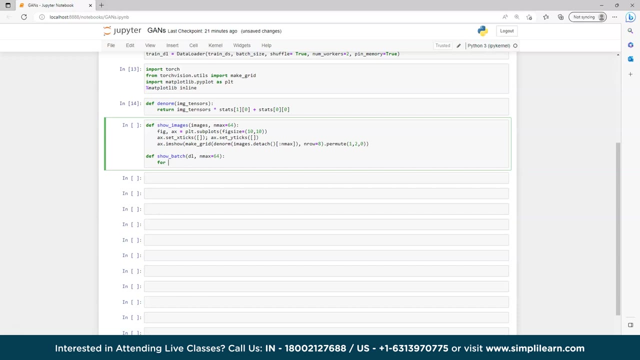 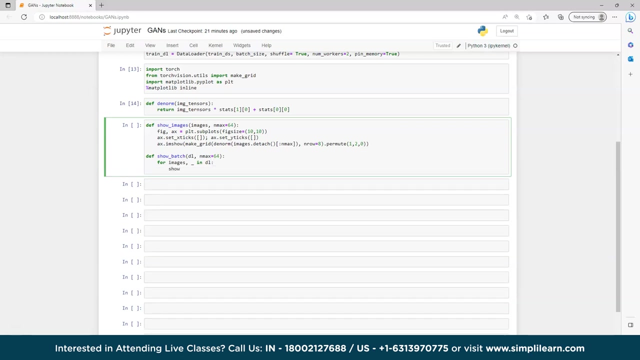 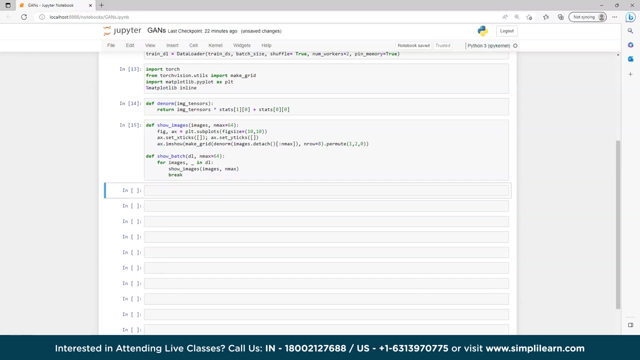 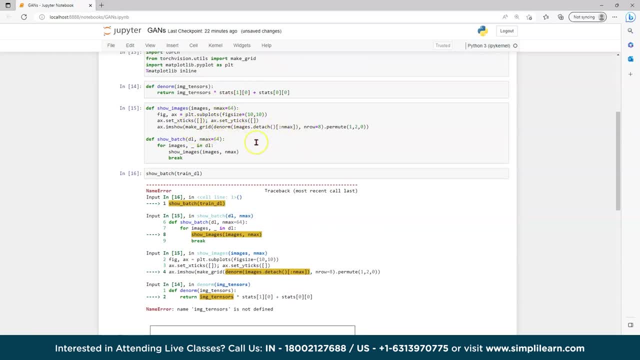 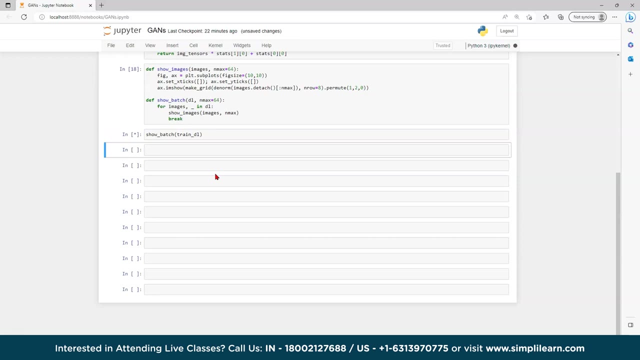 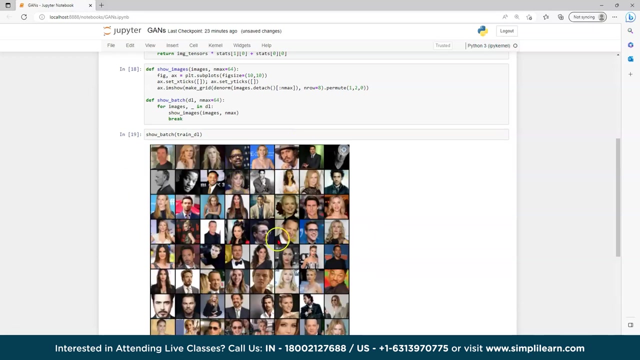 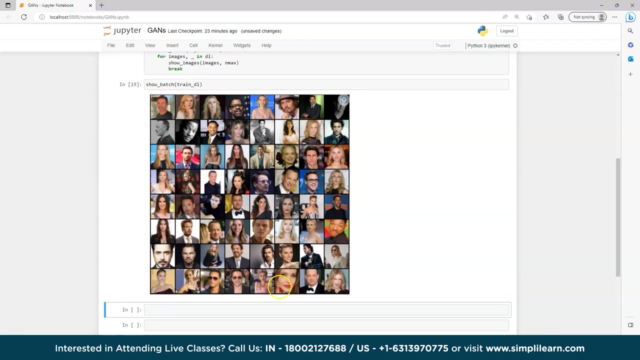 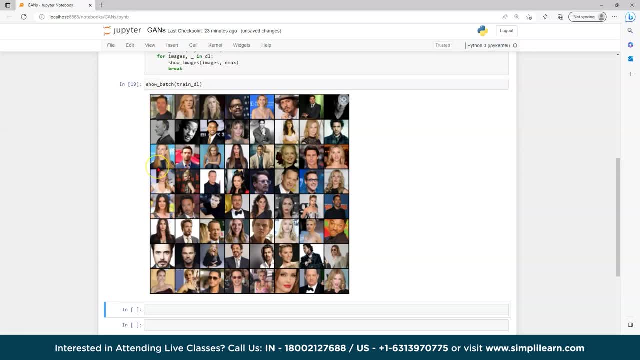 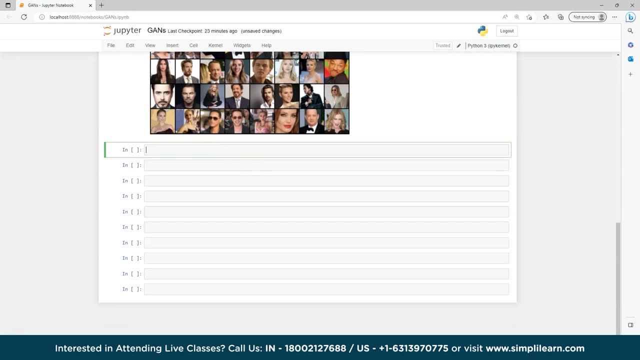 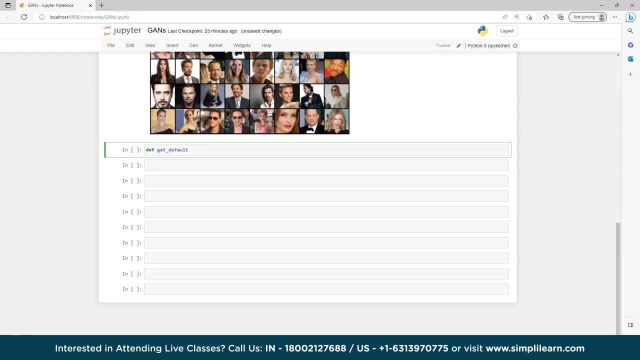 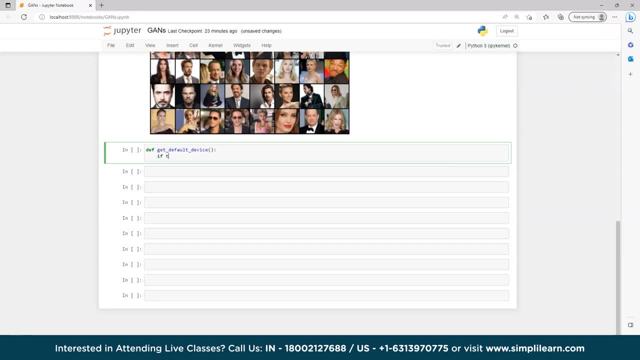 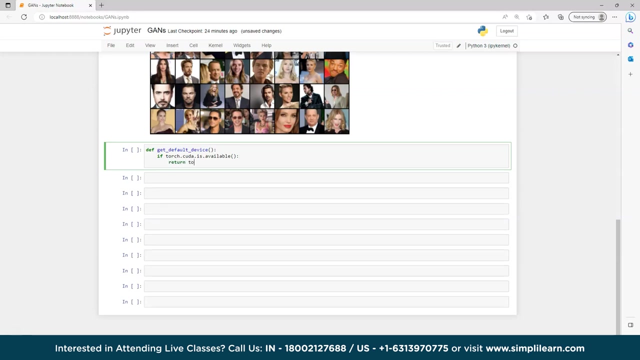 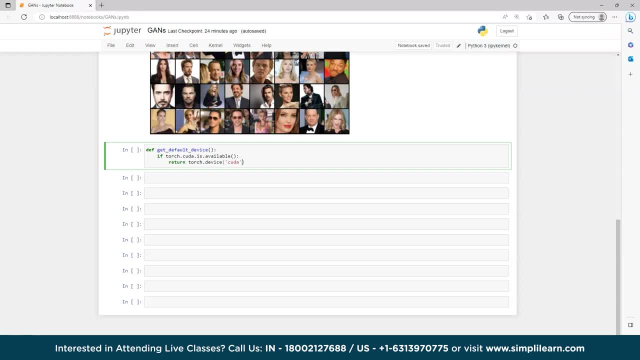 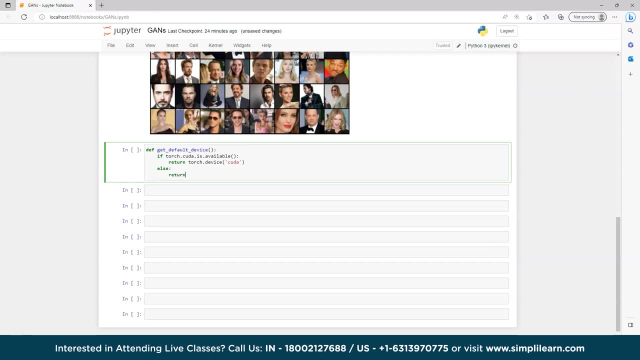 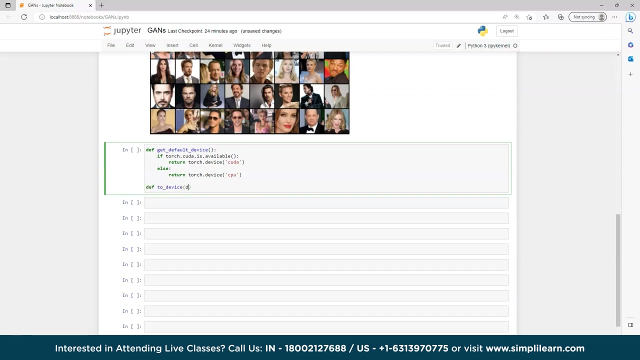 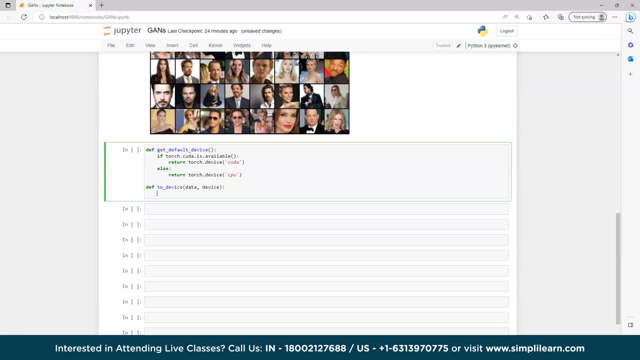 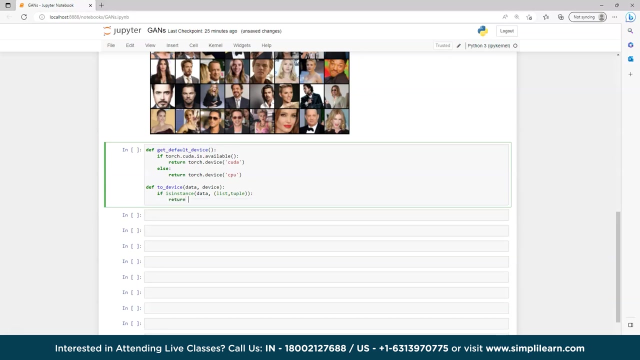 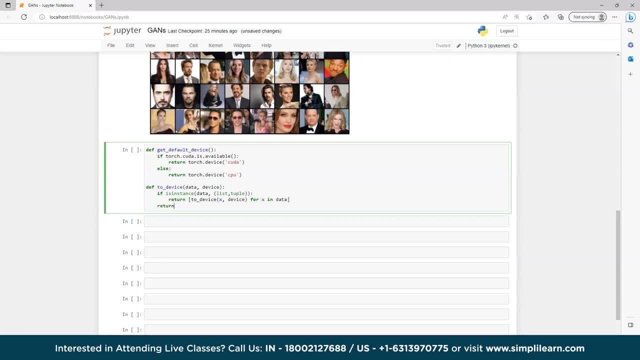 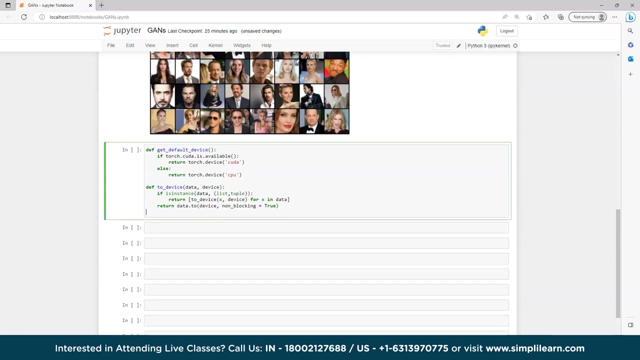 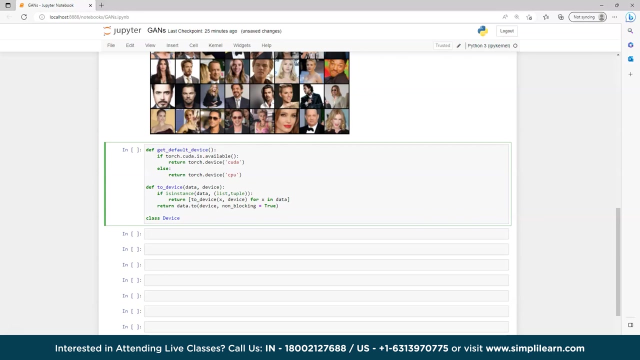 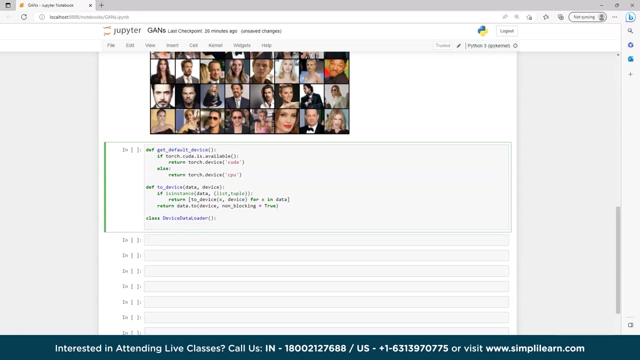 return datato device for non-blocking equals to true. okay, t will be capital here. then I will write class class. class class. i will write dfdevicedataloader. so here what we will do: we will wrap a data loader. 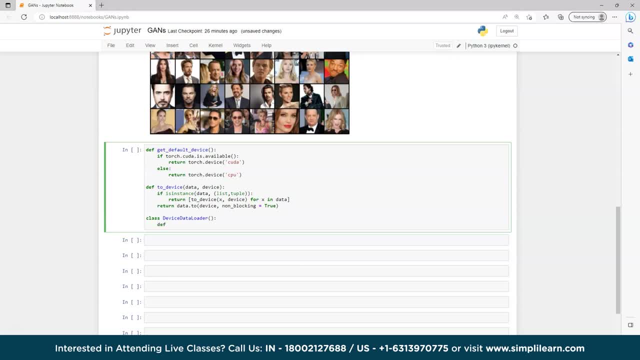 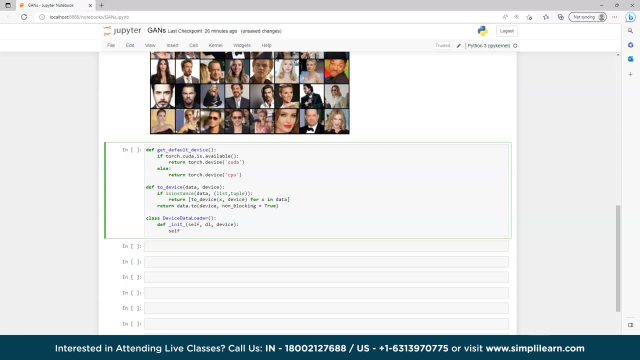 to move data to a device. so for the df init function to self comma dl comma device, then here I will write: self dot dldevice equals to dn. then serve dot device equals device. okay, so here i will write for the iteration. so here i have to give to underscore. 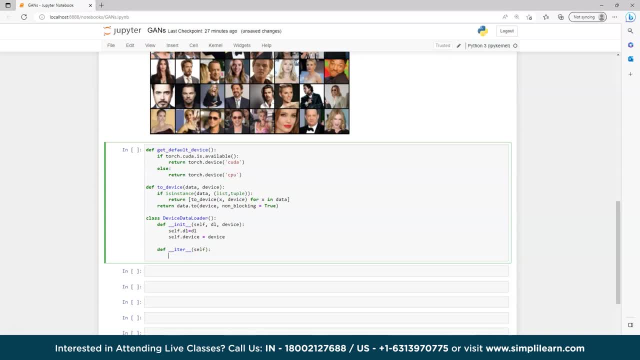 here i will write again self, so it yield a batch to data after moving it to a device. so for, for begin, self dot dl dn, selfdl dn, selfdl dn, selfdl yield to device. then b comma, self dot device. okay, and the last one is df, for the length will write self. 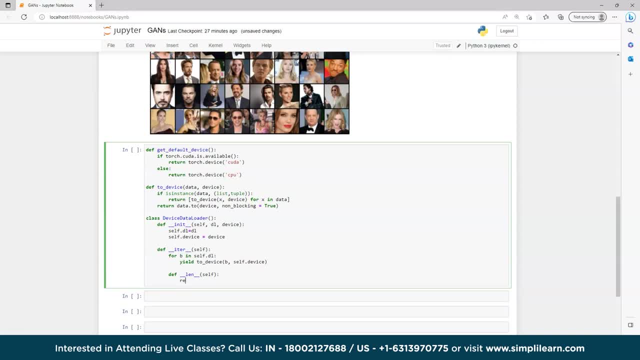 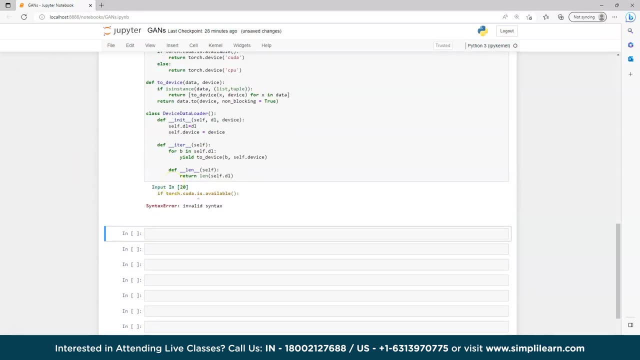 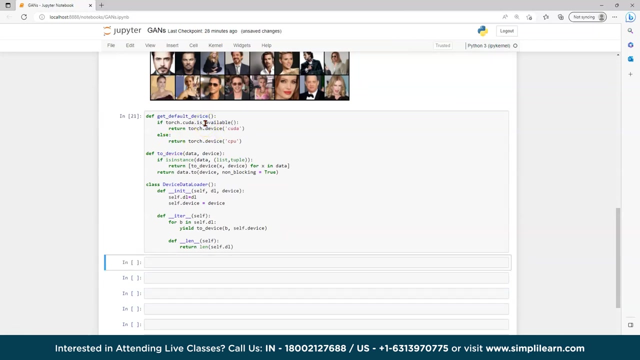 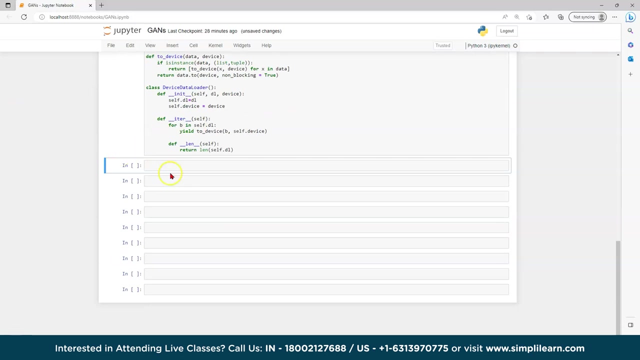 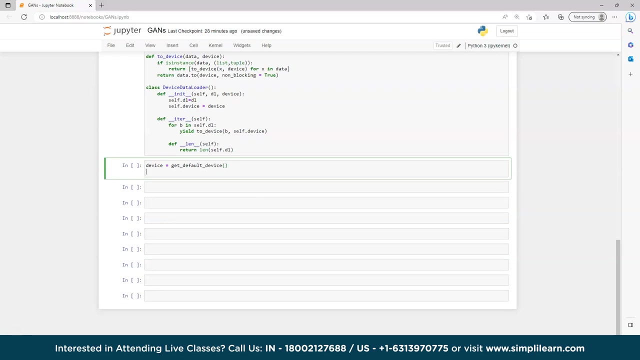 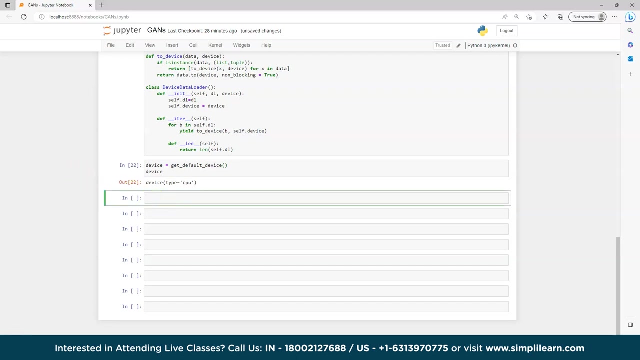 then. then it will return the number of badges. so return length of self, dot, dn. okay, invalid syntax okay, not dot, okay. so here i will write device and i will write device, because you get fault. device device okay, device device okay. place, then play, then then train, then train. 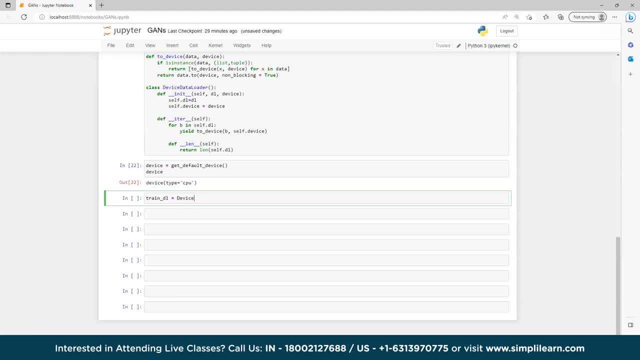 then now, then train, then then dn, then do, then do time device, device, data loader, dl device. already know what is GN and what is discriminator, and you know generator. so let's take again GN overview. so our generative addresses network GN has two parts. so the generator learns to generate plausible data. the generator: 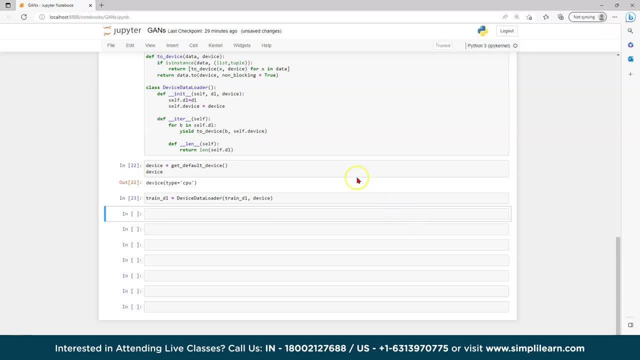 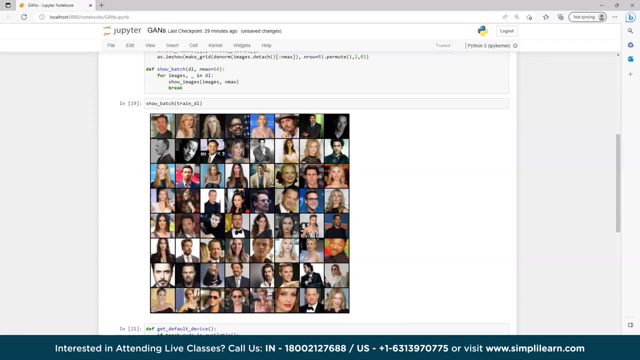 instant become negative training examples for the for producing impossible results. so so you have data. so what discriminator will do? discriminator will, you know, decide from the generated data and the real data which are fake and which are real. okay, this is a generator window. discriminator, sorry, okay. so discriminator, like, takes an image as an input and tries to 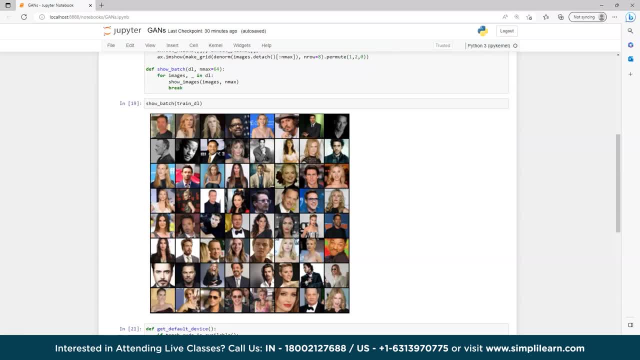 classify it as so. discriminator takes an image as an input and tries to classify it as real or generated, in the sense it's like any other neural network. so i will use here cnn, which outputs is a single neural network for every image. so okay, so i hope you know again like what. 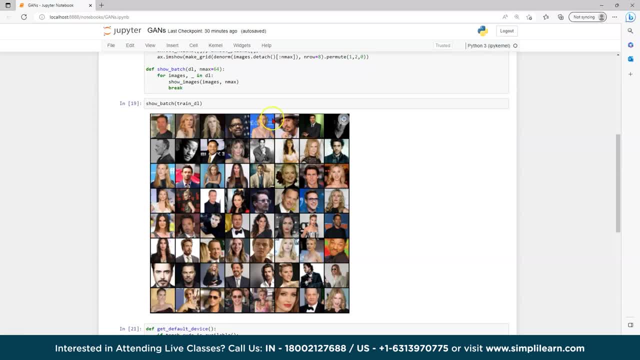 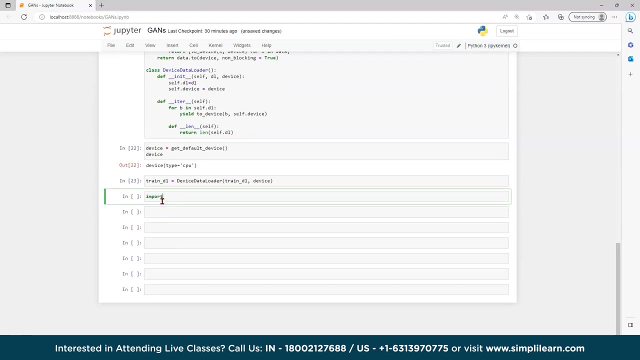 discriminator is, what generator is and what is like real data. it is this, okay, and we will generate the data. okay, fake data and what discriminator will do? discriminator will check whether the data is fake or real. okay, so here i will write import dot dot nn as nn. 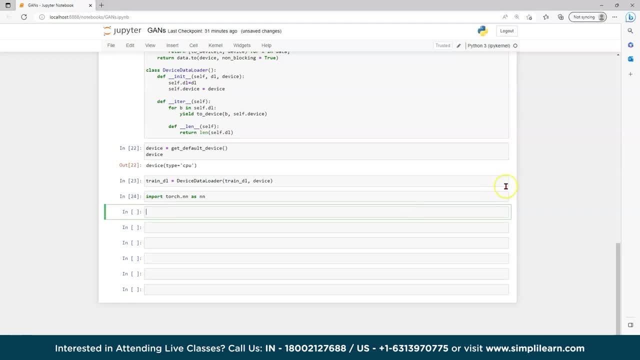 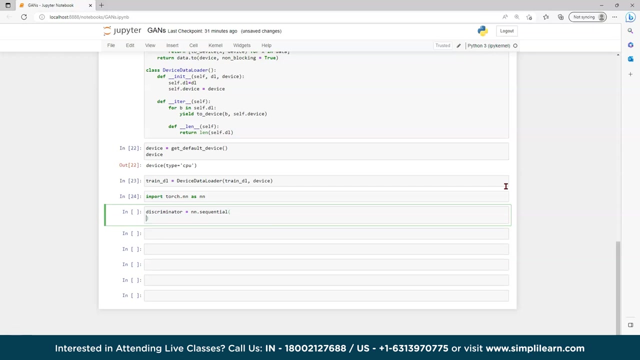 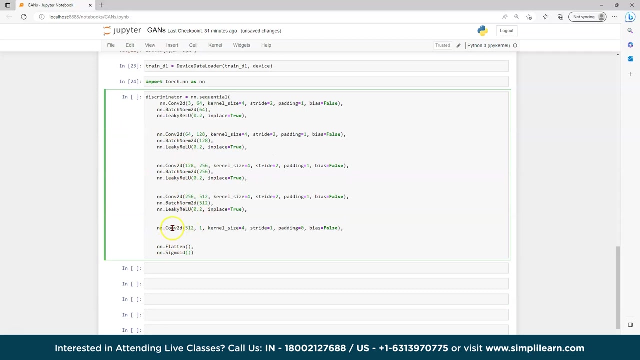 so here i will write: discriminator was to nn dot. sequential. okay, so these are some relatives. ok. flatten layer. convoluted layer: ok, leaky. okay, so here, 64 by 128, 128 by 256. so these are the sizes. sizes of the images, okay so. 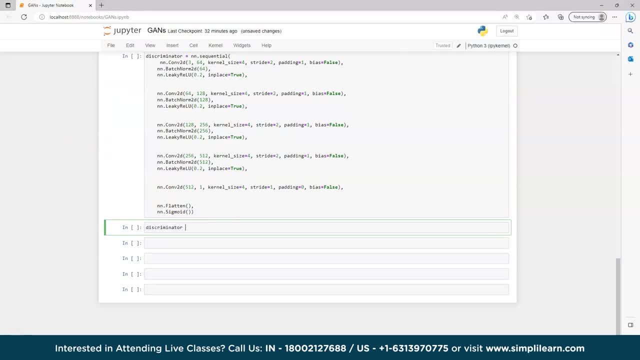 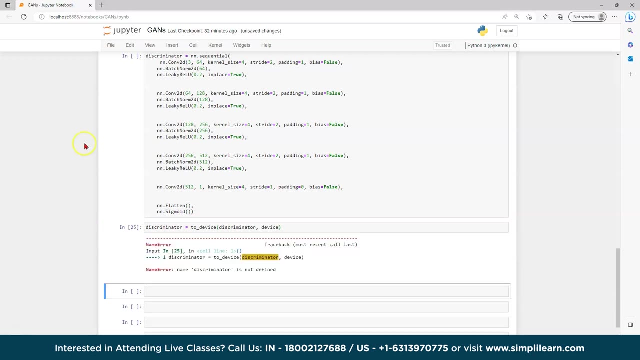 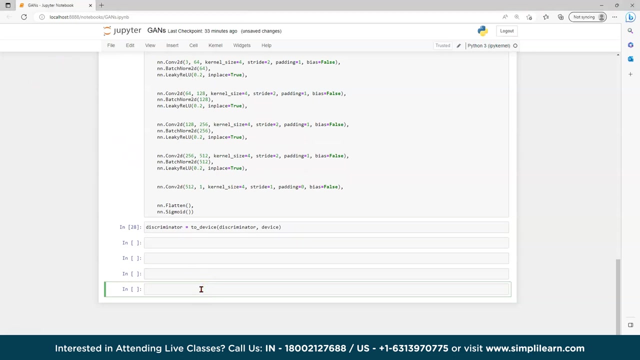 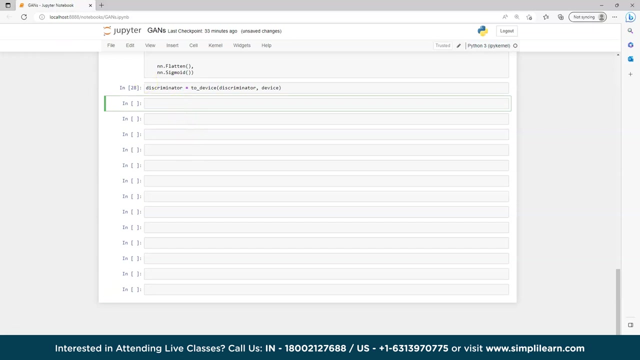 here. discriminator equals to two device, discriminator, comma, device. okay, okay, what's wrong? spelling is wrong, maybe. okay, so it's saying discriminator is not defined. okay, let me debug. okay, nothing else, the spelling was wrong, so sorry for that. so let me do for the peta visuals. okay, so i know, i hope you know the. 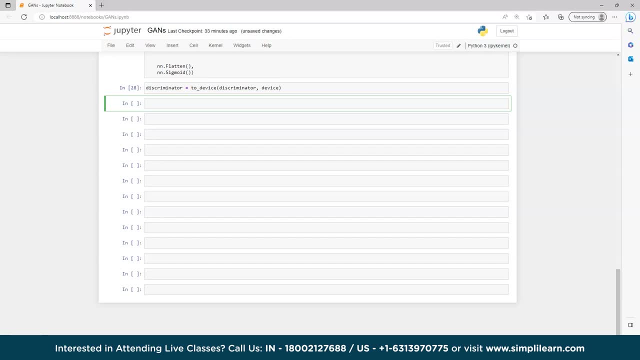 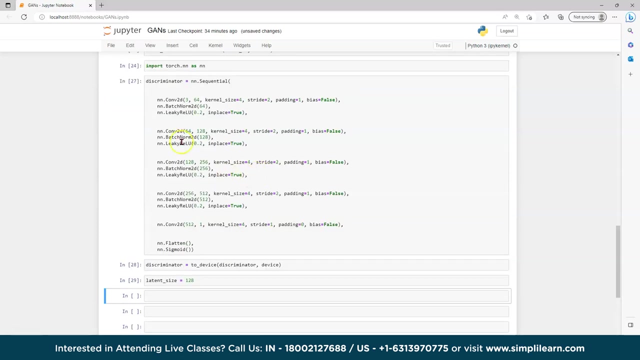 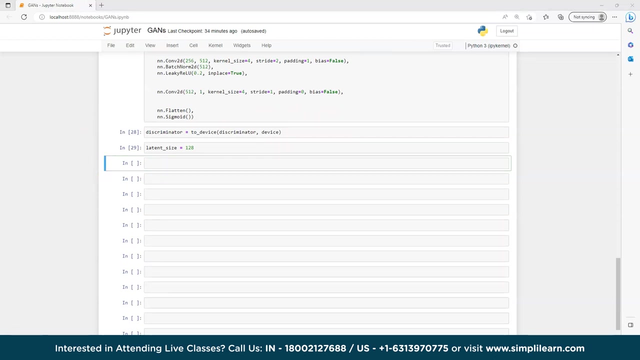 generator, what generator network is so here what i will do: i will set the size. latent size equals to 128. okay, so here we have set this discriminator. now what we will do: we will set the generator, okay, the sizes like three, into 64, 64 or 32, 128 and so on for all the layers. 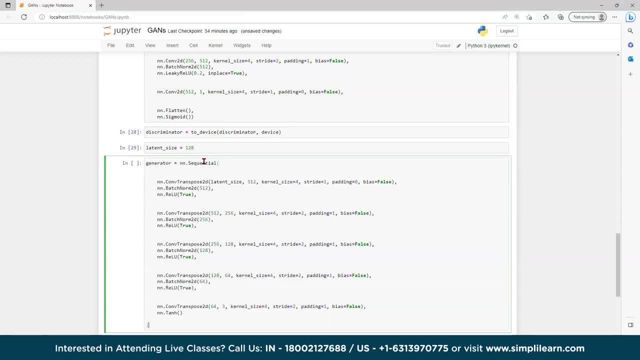 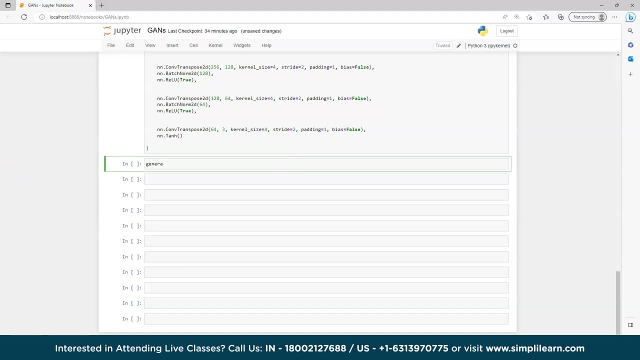 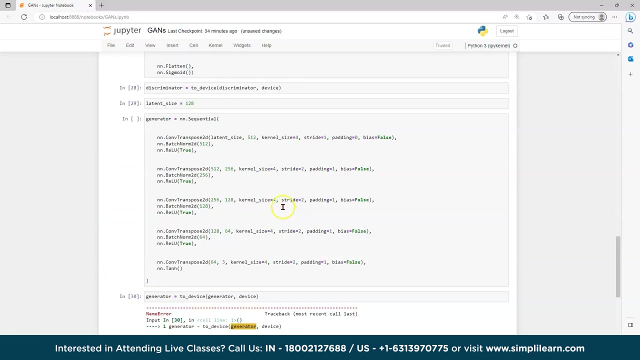 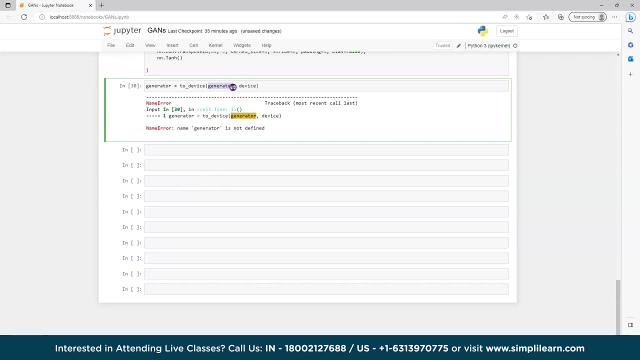 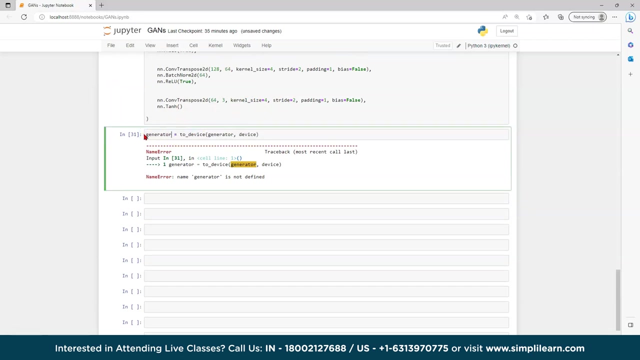 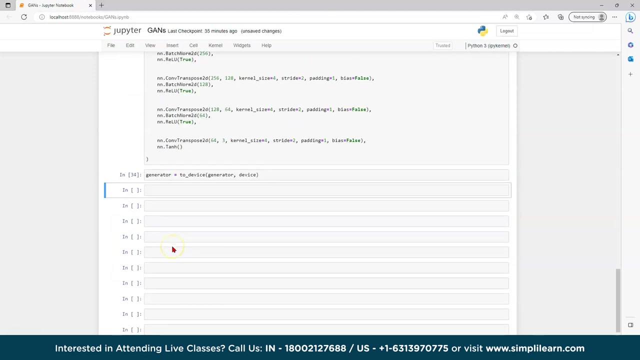 so here I'm setting for the generator the same I will write here, then written for sure to device generator, device, again the generators. okay, then it is defined here. that's working fine, so here. so now what I will do. I will do that is communicator training, okay, so for that I have to write. 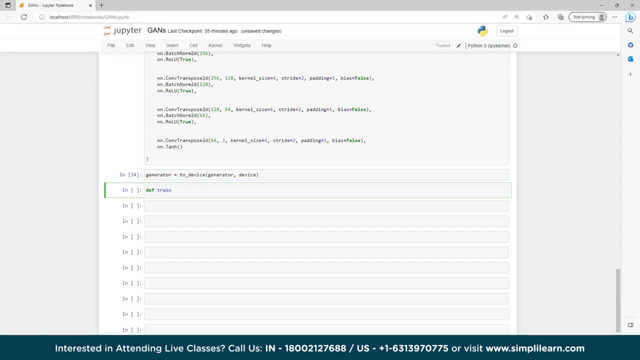 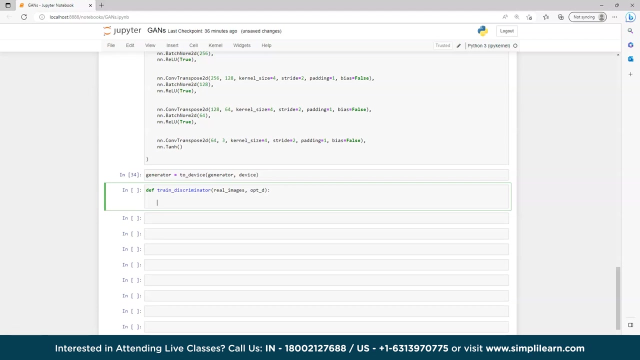 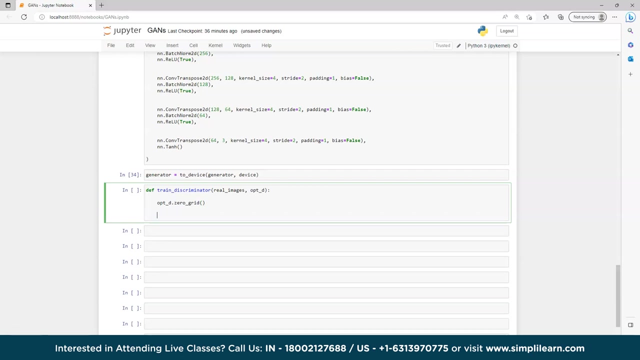 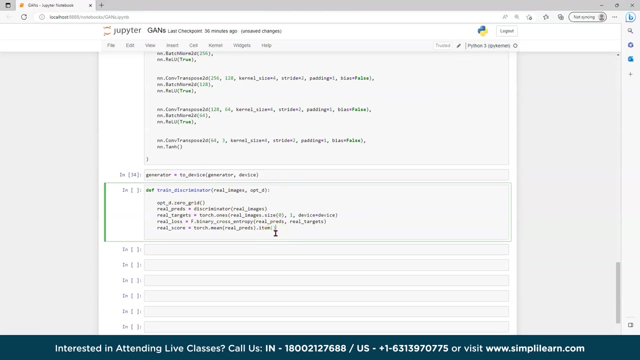 D yes, train discriminator. real images. be okay. now we will clear the discriminator gradients. so opt D dot zero. great, okay, here we will pass real images through discriminator. okay. so these are the for the real images, because why we have to show the all the real and the fake images and we'll shuffle. then I will 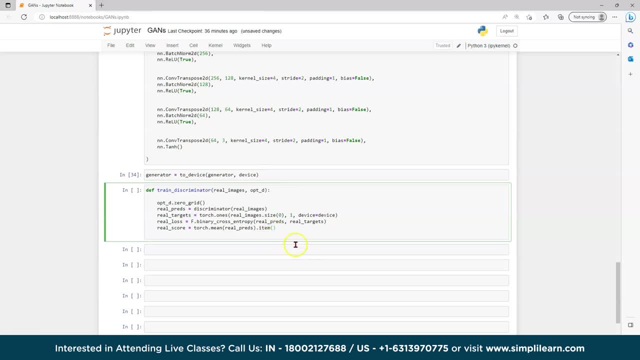 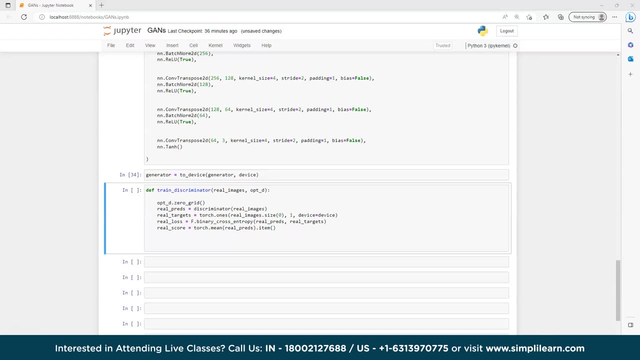 find out which is and which is not okay. so and now we will generate the fake images using latent okay. so for this later it equals to torch dot random input and the best size we are giving- the latent size we are giving okay fake images- is called the generator. 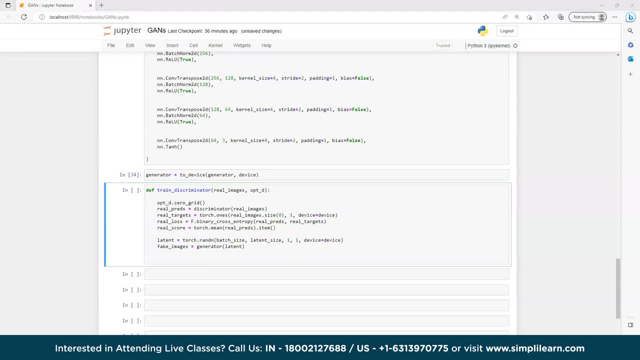 okay, so now what we will do. we will pass the fake images through discriminator, as we did for the real images. okay, so now we will update discriminator weights. for that i have to write: loss equals to real loss. then plus fake loss: okay then loss dot backward, opt d dot step. 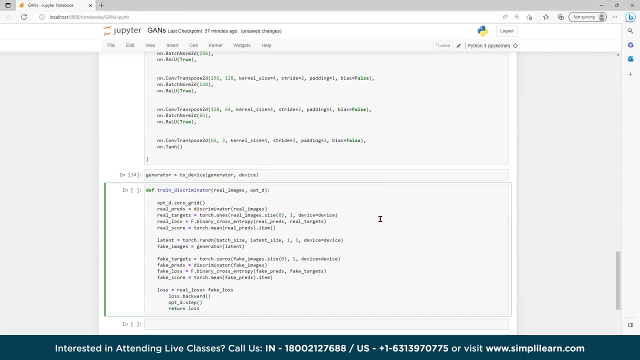 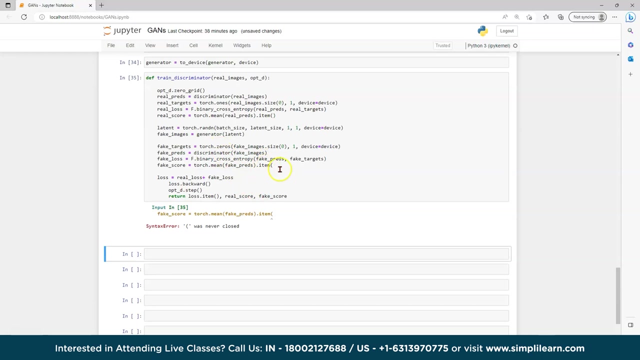 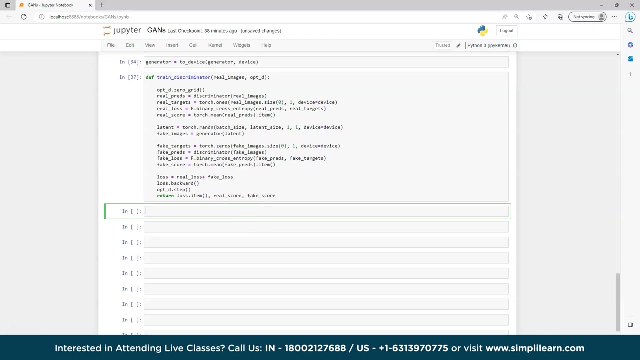 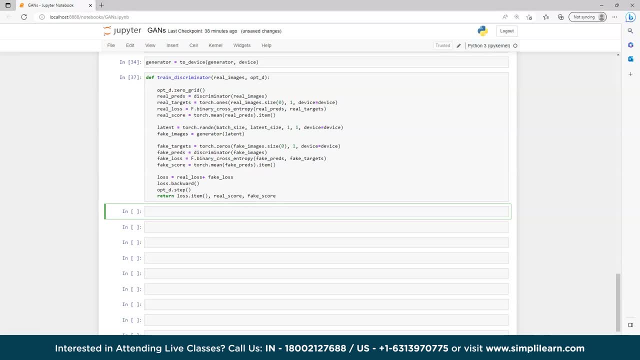 images and at the same time, we pass the fake images through discriminator and the at the end that laws equal to real laws and the fake laws. we update the discriminator weights. okay, so now. so this was the discriminator training. now what we will do, we will do the generator. 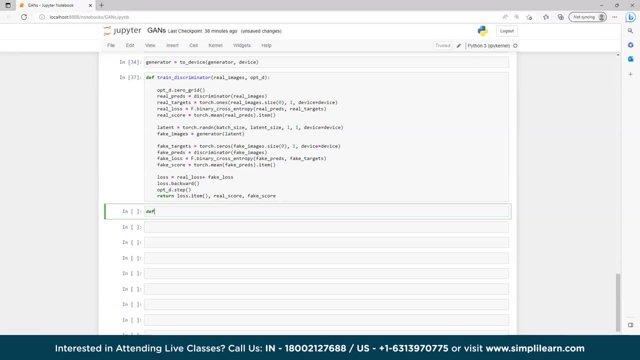 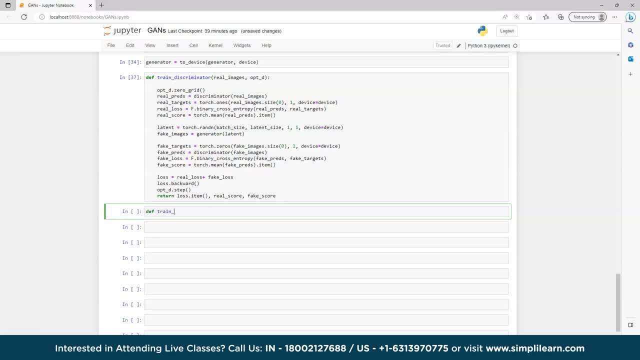 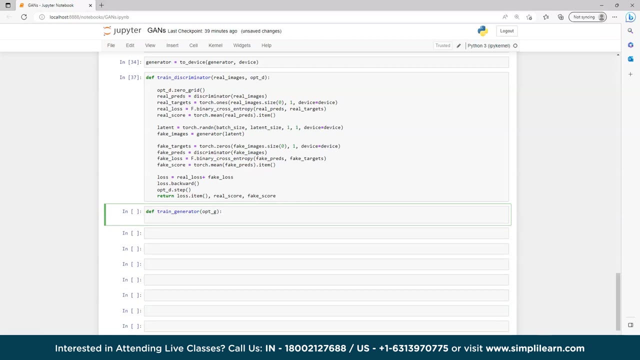 for that i have to write def: train generator, generator, then opt g, then opt g, then opt g, dot, dot, dot, zero, zero, zero, red, red, red. so what we are doing here, we are. so what we are doing here, we are. so what we are doing here, we are clearing the generator gradients. 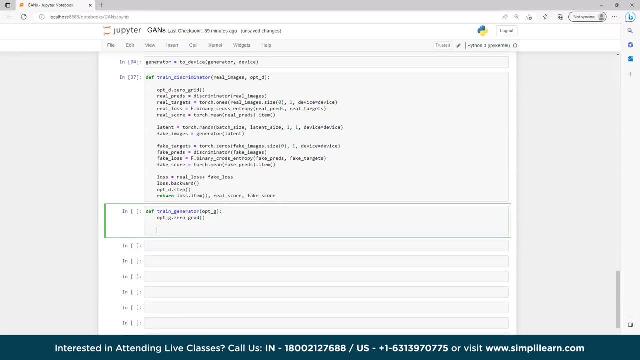 clearing the generator gradients. clearing the generator gradients. before that, we did for the same, the before that, we did for the same, the before that, we did for the same: the discriminator, one, discriminator, one, discriminator, one. okay, so now we will generate the fake. okay, so now we will generate the fake. 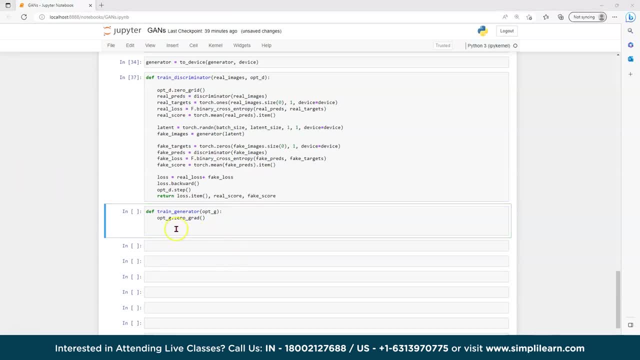 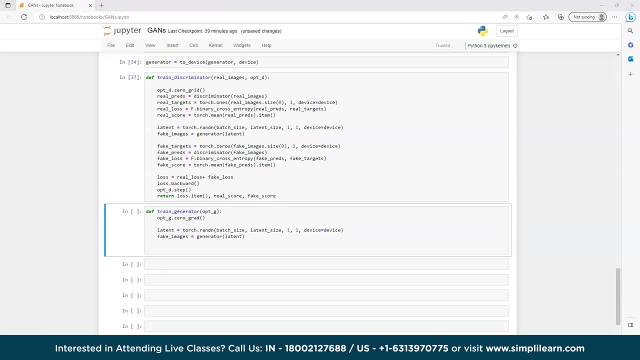 okay, so now we will generate the fake images, images, images. okay. what generator do? generator only? okay, what generator do generator only? okay. what generator do generator only? uh, generate the fake images. uh, generate the fake images. okay, okay, okay, so, from so, from so, from this prediction, this prediction. 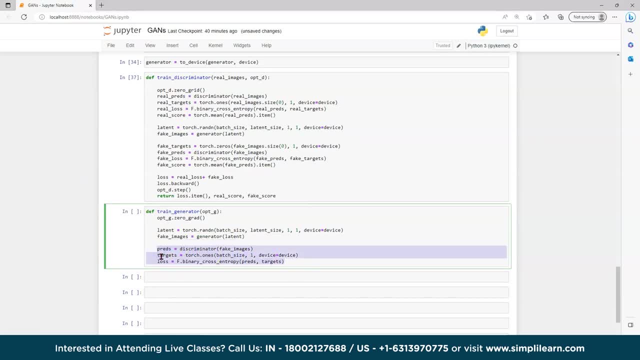 this prediction, from this prediction, what we are doing, we, from this prediction, what we are doing, we, from this prediction, what we are doing, we are just make trying to fool, the are just make trying to fool, the are just make trying to fool the discriminator, discriminator, discriminator. okay. 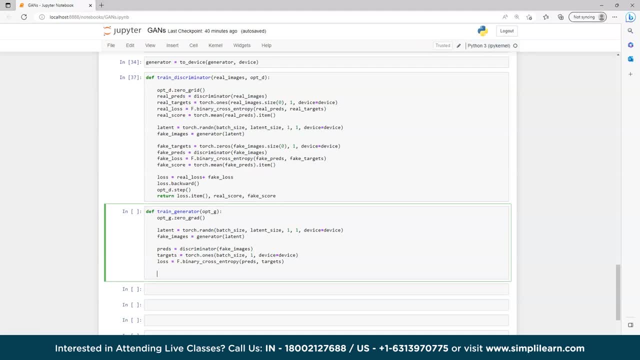 so, so, so. so here we will update the generator. so here we will update the generator. so here we will update the generator. weights: so i will write loss dot weights. so i will write loss dot weights. so i will write loss dot backward, then i will write opt. 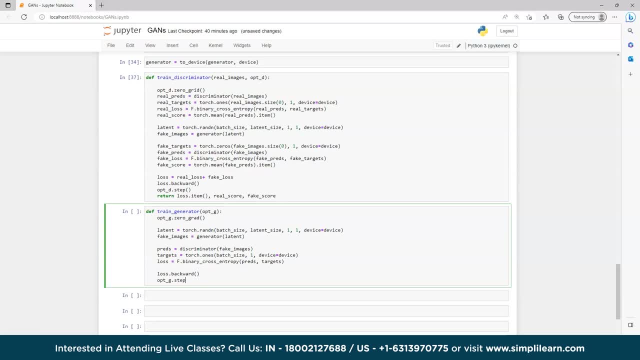 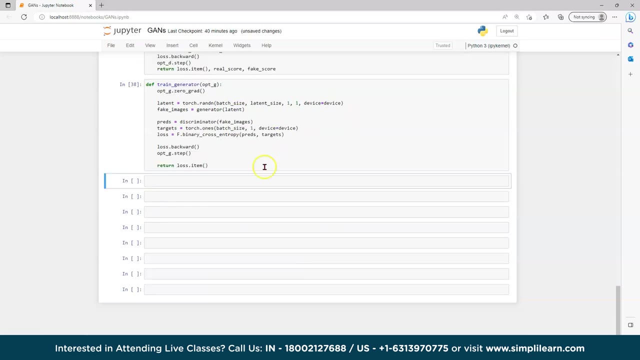 then i will write opt, then i will write opt: underscore g, underscore g, underscore g: dot step. then here we like return loss, then here we like return loss, then here we like return loss item. okay, let's run it. so here i write from. so here i write from. 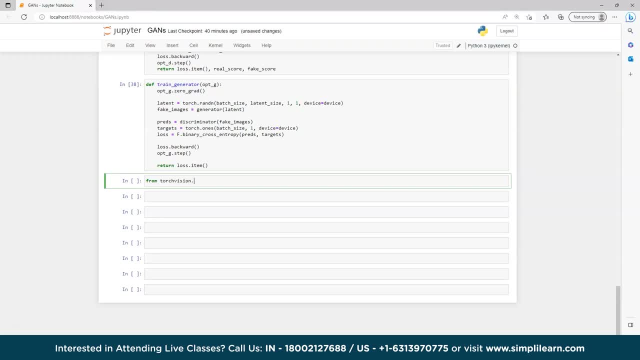 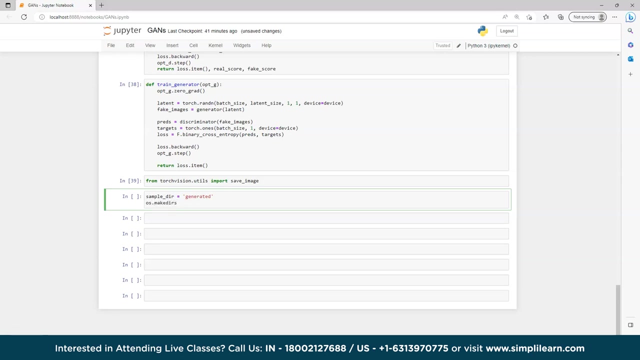 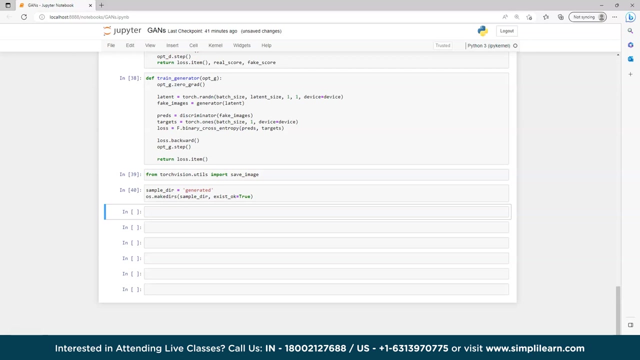 so here i write from torch torch, torch, vision, vision, vision, dot dot dot utens, import, save image. and here i will write sample directory because generated, generated, okay, and osme directory, sample directory, comma exist, okay, true, okay. so now what we will do? we will save the sample data, okay, so we, i have to create, uh. 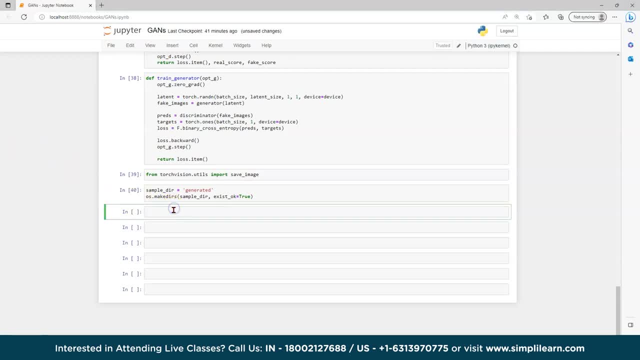 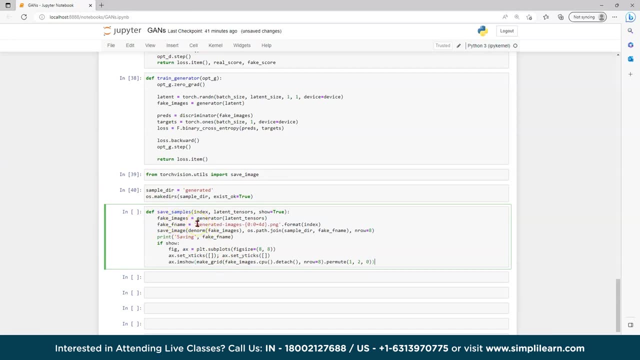 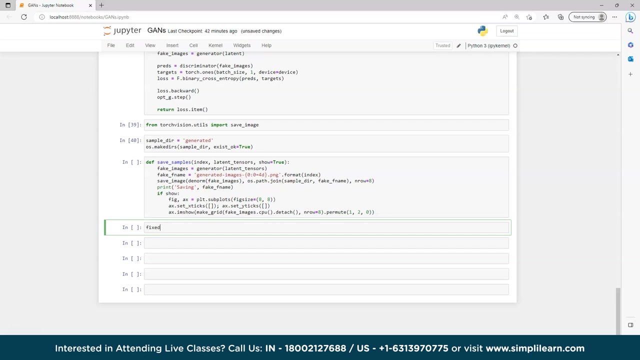 to save samples. uh, one function, okay. so here what i'm doing: we are i'm making the fake images, generating the fake images and saving it. okay, so moving forward. but what i will fix? the? i will fix the latent. latent equals dot, dot, random input, then 64. 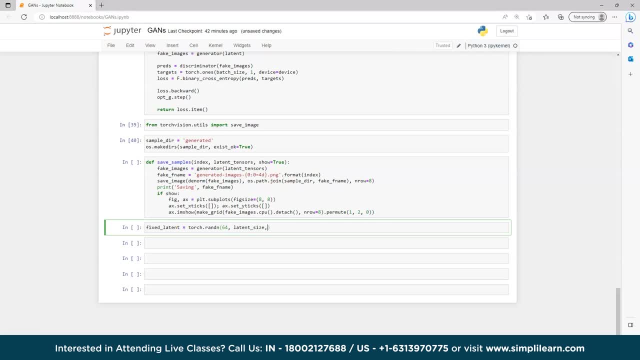 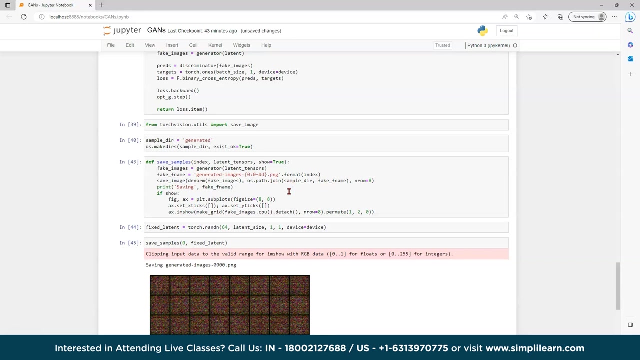 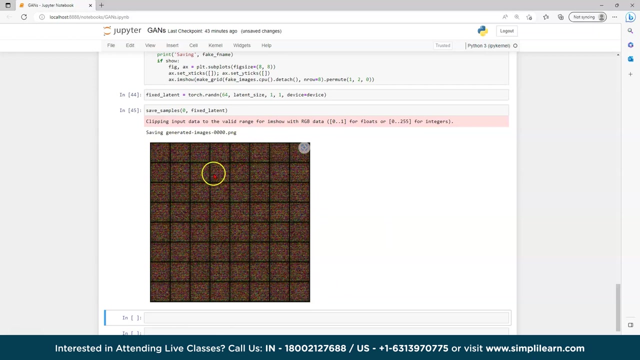 latent size: comma one, comma, one comma. then device question: device. then again save samples to zero fixed latent. okay, save samples is not defined. it's defined here. yeah, so see, this is the generated images. this is a fake image. okay, now what i will do. i will do the full training loop. 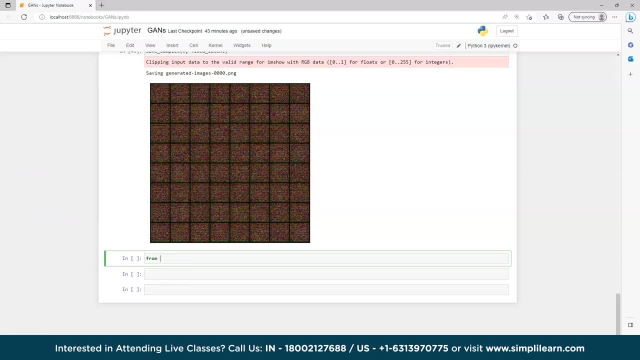 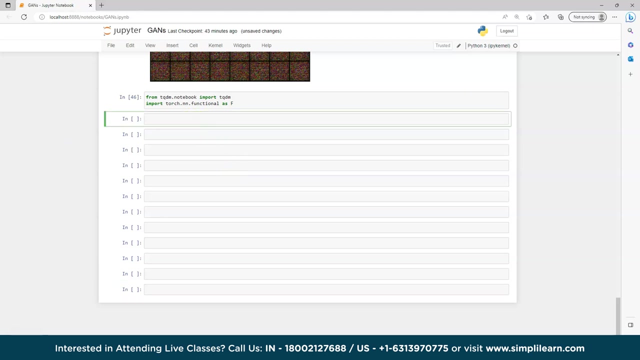 for that i have to write from tqdm dot notebook import tqdm and import dodgennfunctional as f. let me give the spaces. so now what we will do. we will train this. uh, we will do the full training loop till the 400 epoch. so it will take a. 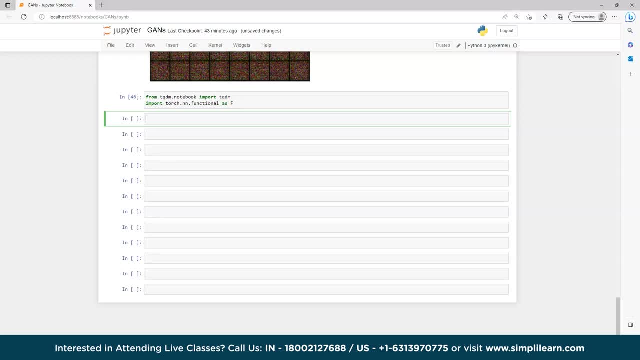 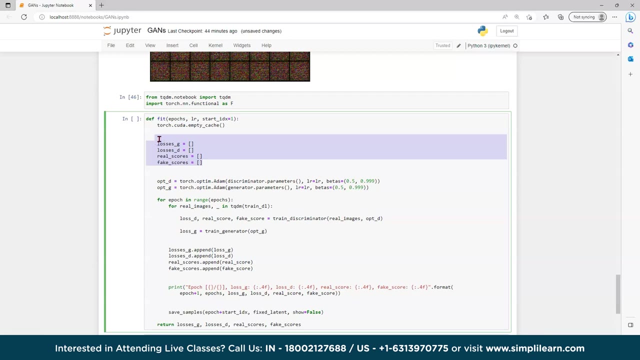 very long time. so first i will write the definition, okay, i will define one, uh, the function, okay, and then i will get back to you. so yes, what i did, uh, so this, i have set the losses and the scores and the scores, okay, and these are the optimizers, some optimizers, obt. you can say: 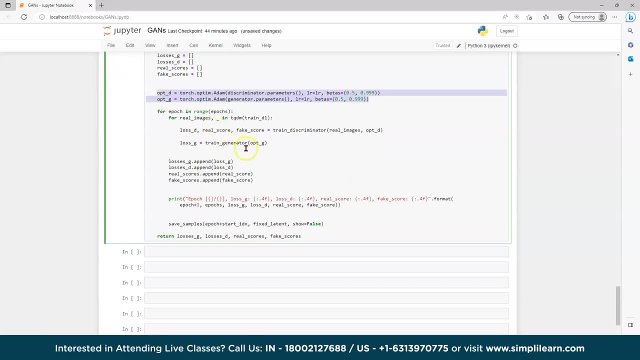 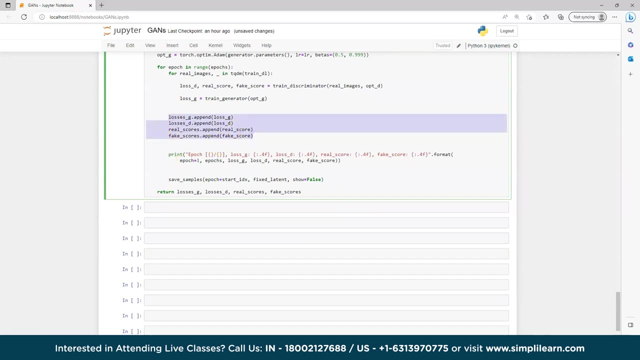 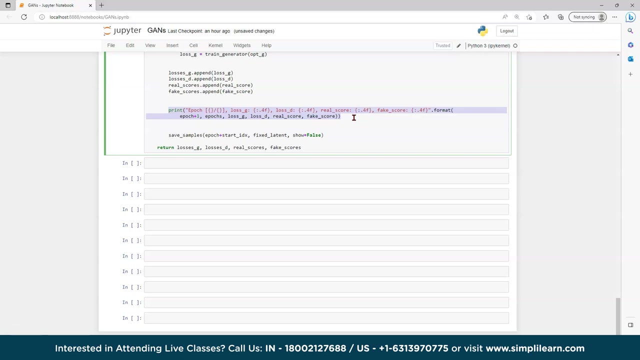 optimizer we are creating, and here i am training the uh discriminator and here i am training the generator. okay, for the loss, and here the record of the loss in the you know scores will save, and this is for the log of losses in this course, last batch, and for this. this is for the generated image. okay, it will save the. 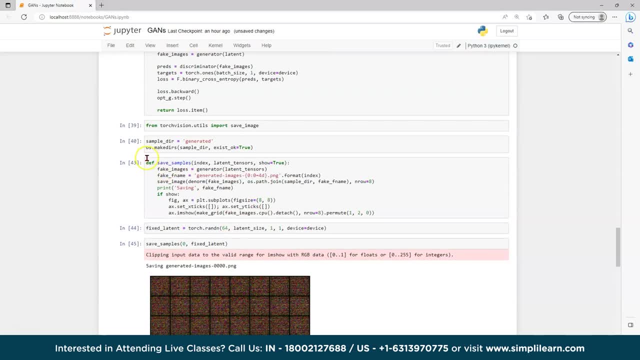 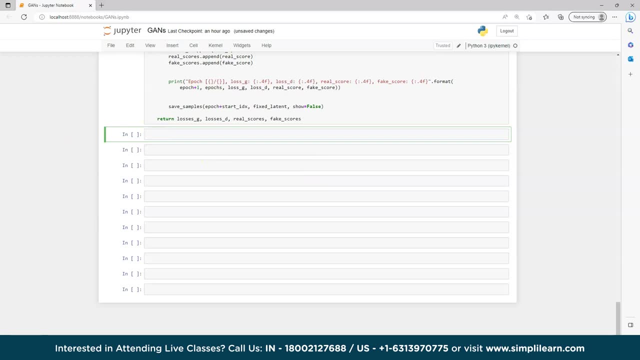 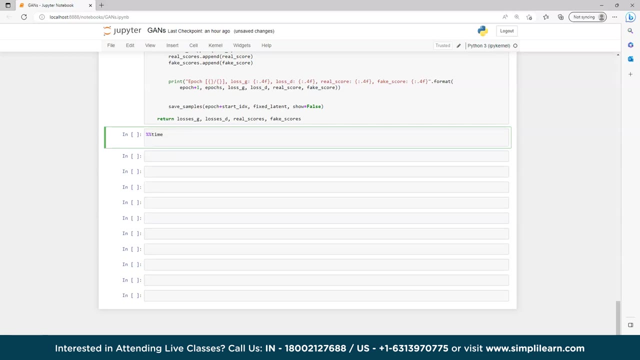 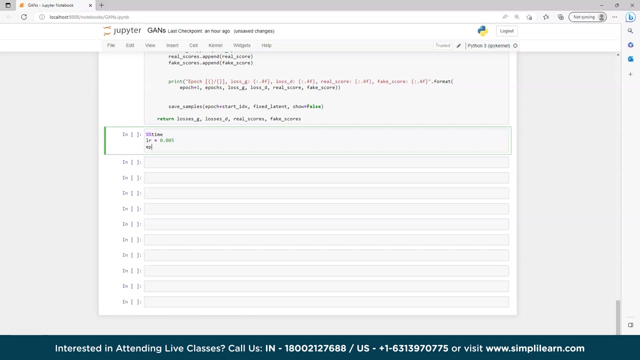 generated image. okay, we have already created here you can see for the sample image, for the saving. okay, now what i will do. i will write percent, percent time. then lr equals to 0.005, then a box equals to 400. a box means it will take a huge time. so history equals to fit. 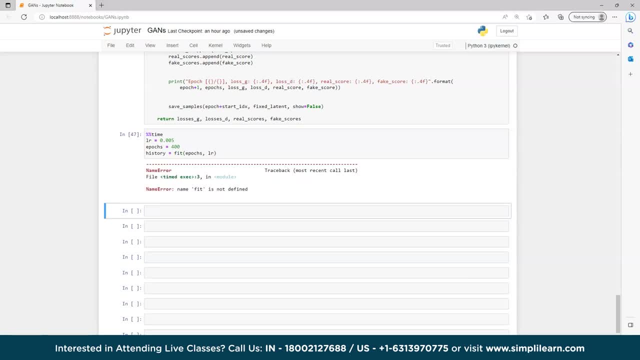 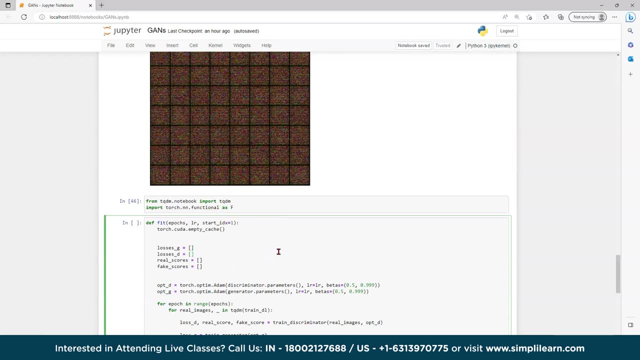 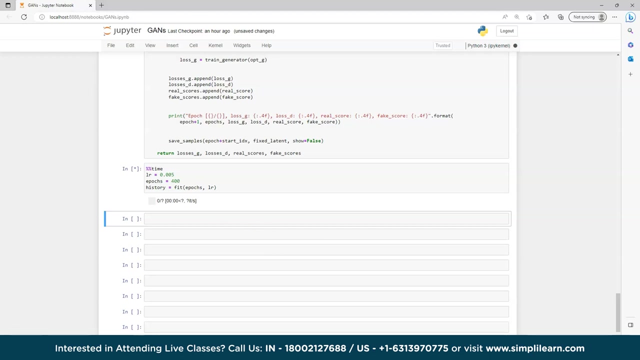 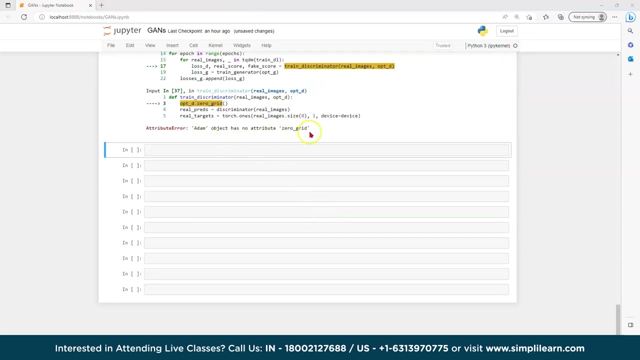 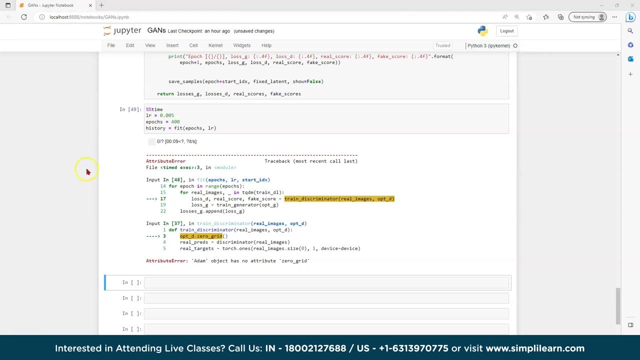 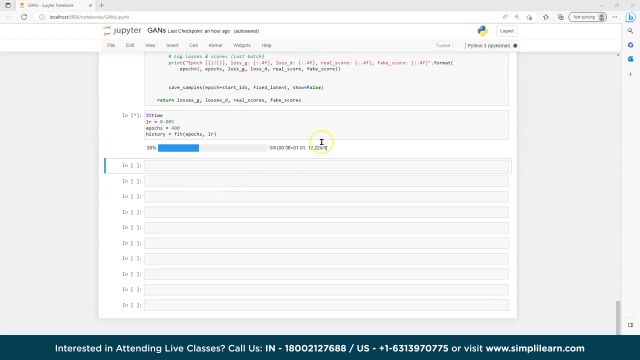 a box, okay, if it is not defined, okay. okay, why it's coming like this. okay, something other item object has zero grid. okay, check. so, as you can see, it has started running. so this box will run till 400. so it will take a long time, very long time, so i will get back to you after that. 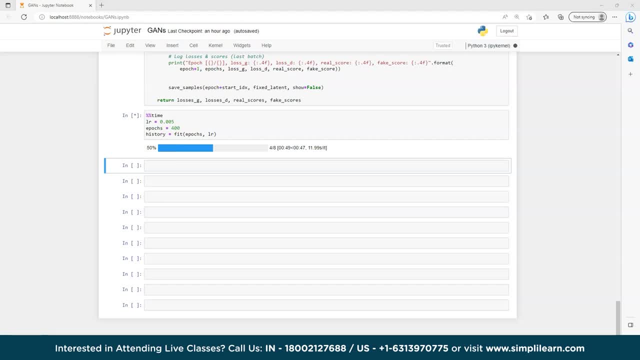 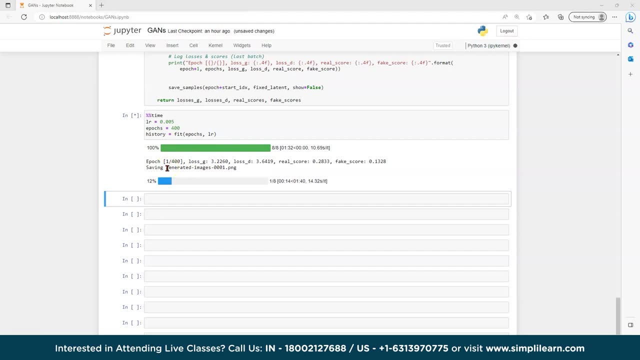 so, as you can see, this is a 1 by 400 box. you have to believe me, on the ass ebox hundred, so it will run to three till 339. okay, so it will take a very, very long time. so it will define the loss of generated, the loss of discriminator, and the real score and the fake. 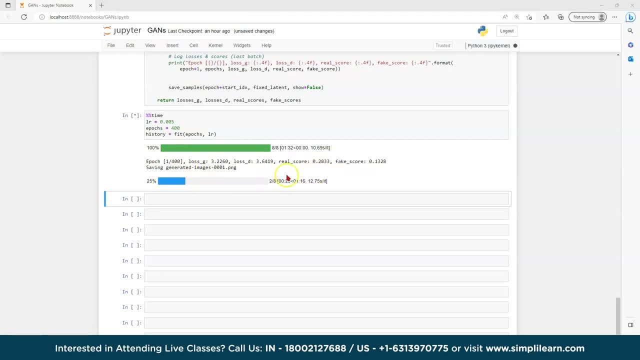 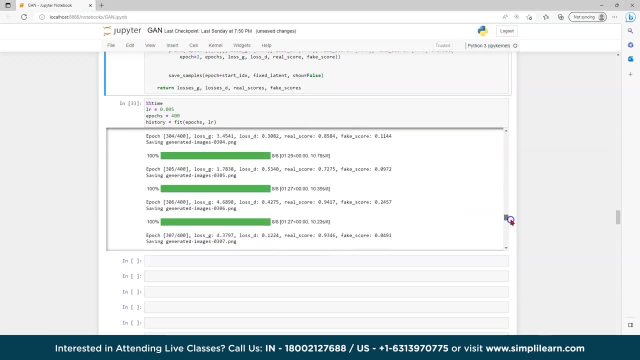 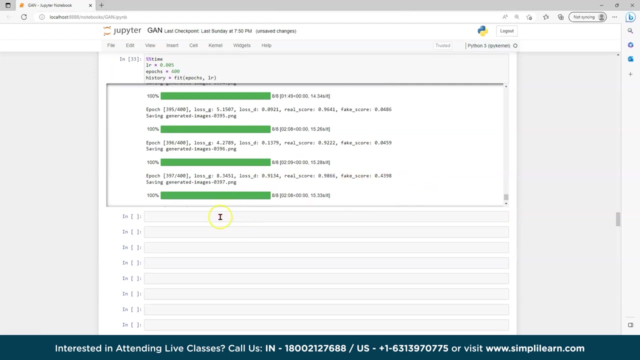 score and at the same time it's saving the generator images, okay. so it will take a long time and then i will get back to you. so, as you can see here, the gans are done till like 400, okay, till all the 400, okay. so now let's do some losses, common losses of discriminator and the real score. 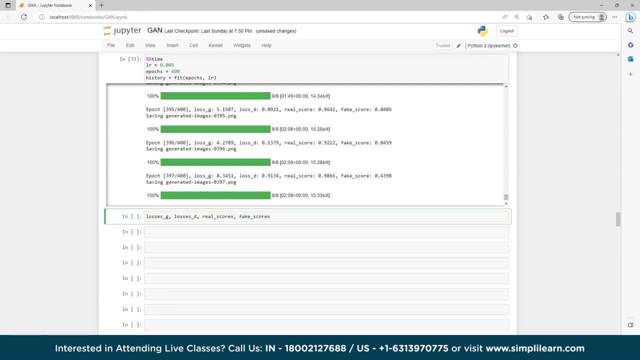 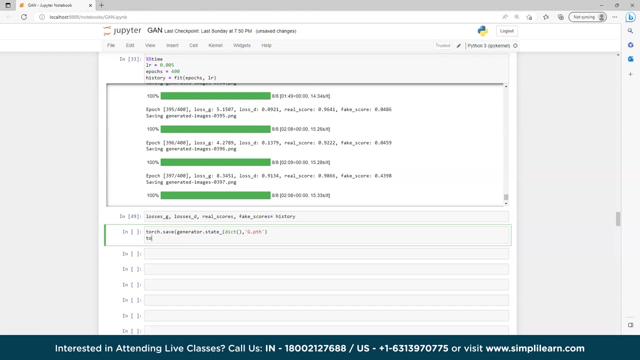 and the fake scores question history. so here i will touch dot: save the generator dot state. let's go directory path: comma g: dot path. okay, then i will write dot, dot save the discriminator dot state. directory path: comma d: dot. ptr, dot h. okay, so my spelling mistake is there. 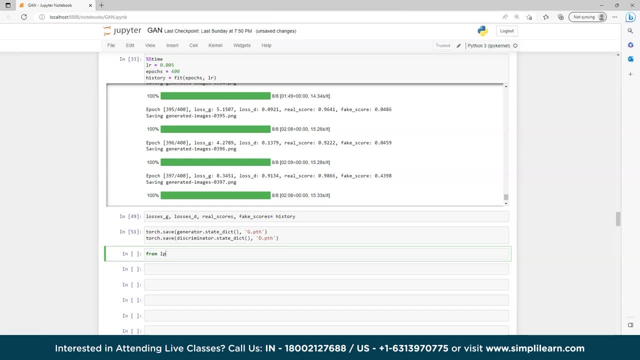 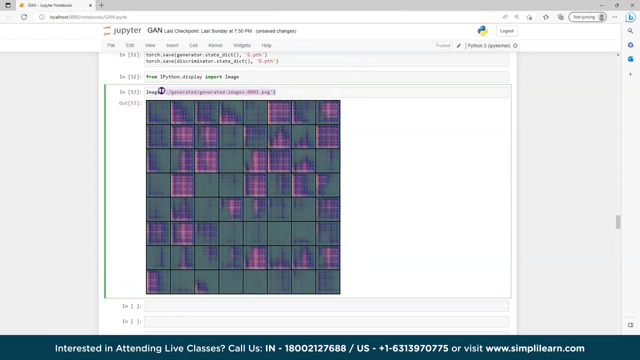 yeah, so i've read from ipython dot display import image. okay, so here i will write image like what the generator generated. the image dot slash generated slash Notepad image images. this is the first image have generated by the generator. okay, so same. we are 400 a box, so let's. 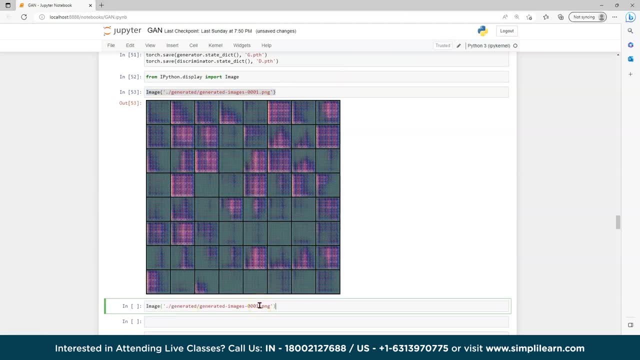 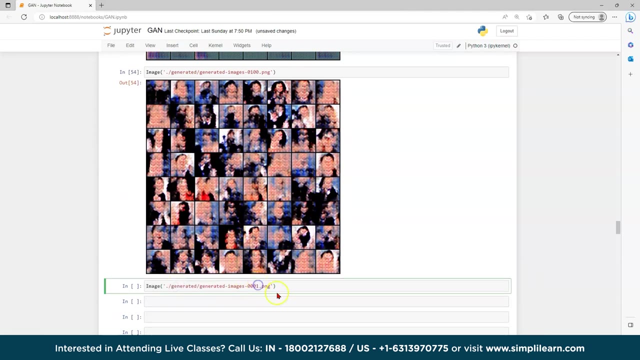 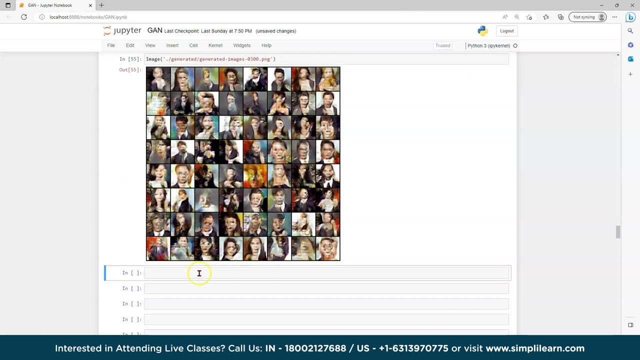 see The table's erased, swept, all all. So here I will check the hundred image. So, as you can see, hundred image is more bit clear. So what if I will check for the like three hundred in three hundred image one? It's more bit clear. Okay, Now let's check the four hundred image.